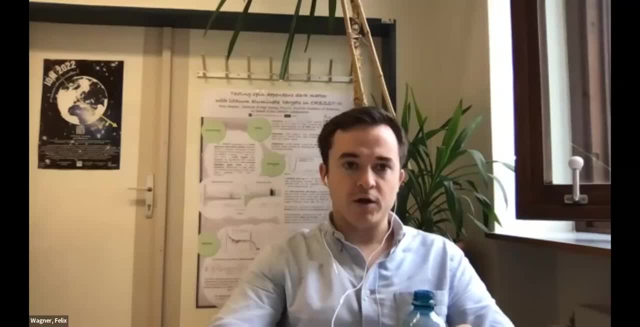 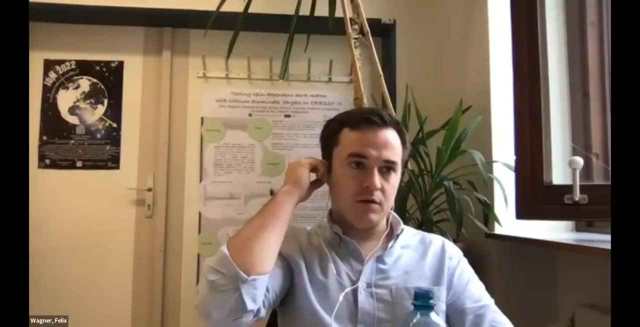 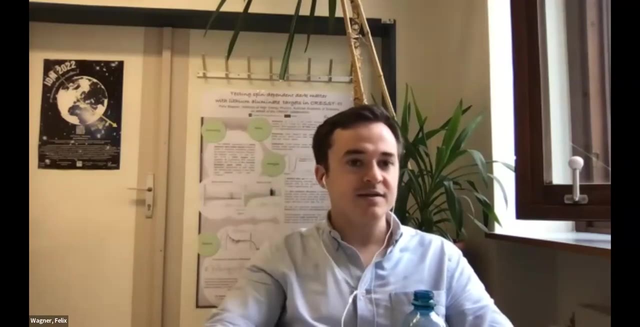 there is no strict limit, So don't you worry. if you overflow the time or you make it too short, Doesn't matter. Yeah, Okay, Yeah, I planned for this one hour slot and to allow some questions in the end, but that's okay, Then I can go relaxed in some. 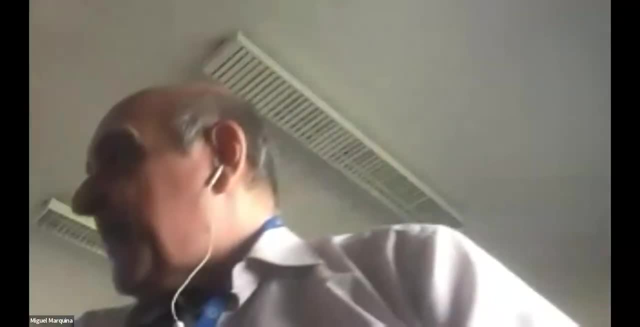 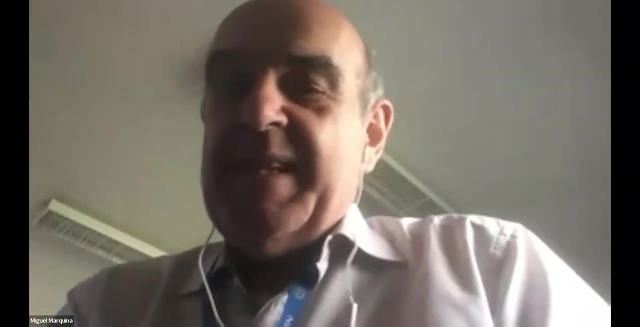 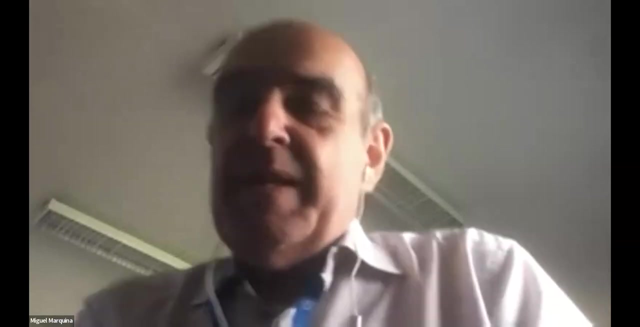 that's okay. I think it's 11 past now, but let's go for it. Anyway, I am going to have a couple of minutes in just saying small things, So okay. So, good morning everybody. Thank you for joining us to this new delivery issue of the QTI lecture program, And today we are 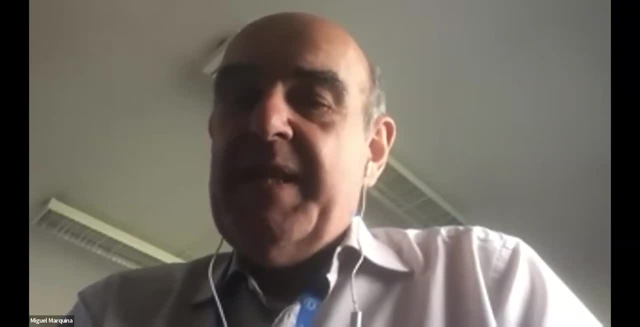 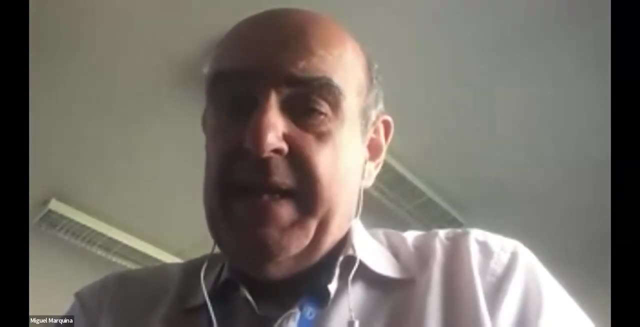 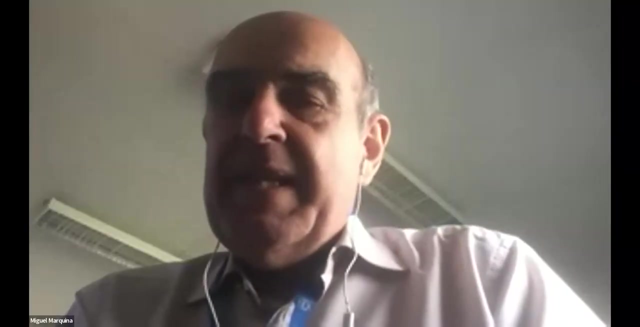 happy to host Felice Wagner from the Austrian Academy of Sciences- Actually from. you are working, if I understood well, directly in the HEPI High Energy Physics Institute, where you are doing your PhD. So now, before giving the floor to Felice, let me just remind you. 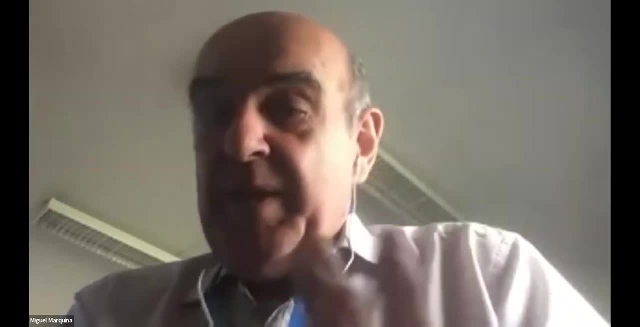 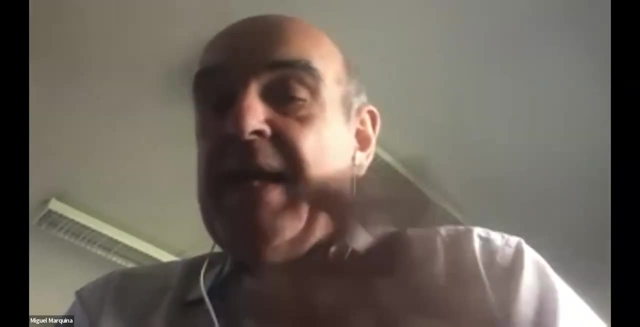 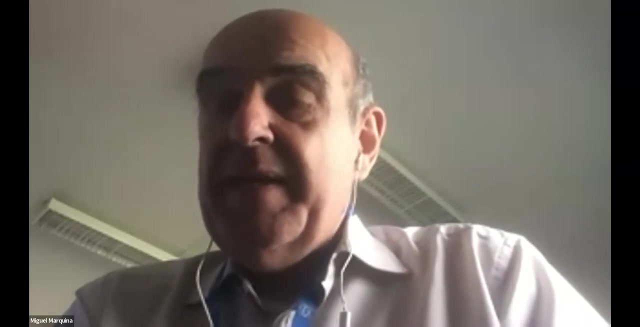 of a couple of points. One is that we are recording, as you have noticed by now, because you have to accept it. We are recording this lecture. So, in the event that either you want to replay or, maybe even more useful, that you know of colleagues that couldn't make it today, 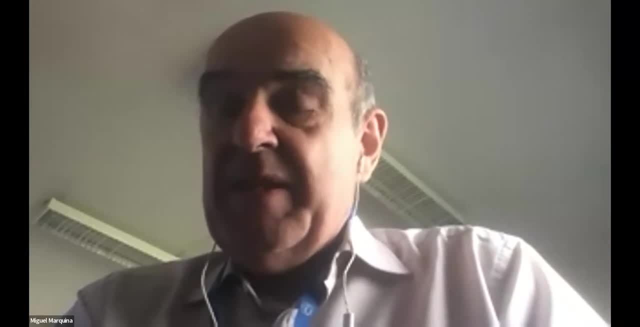 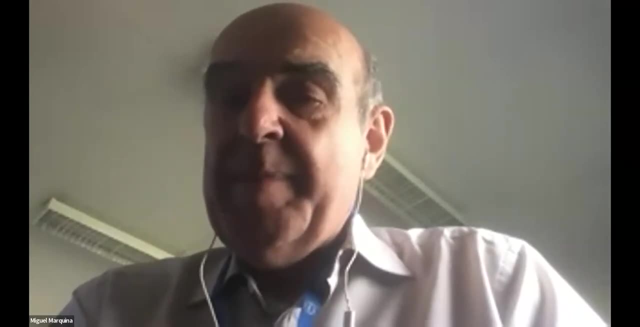 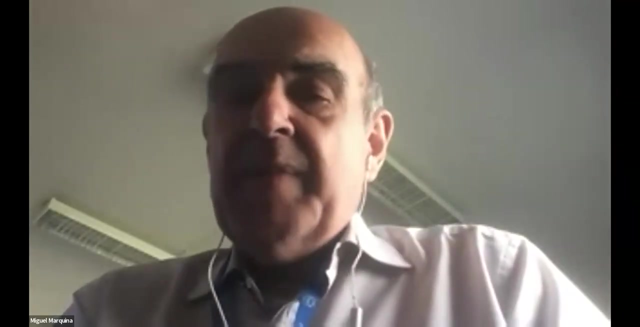 the live presentation. just know that this presentation is going to be uploaded into the IndyCo website, where you have found the reference for this lecture, And you can play it again offline at your ease. Another thing I didn't share with Felice, but if he offers, 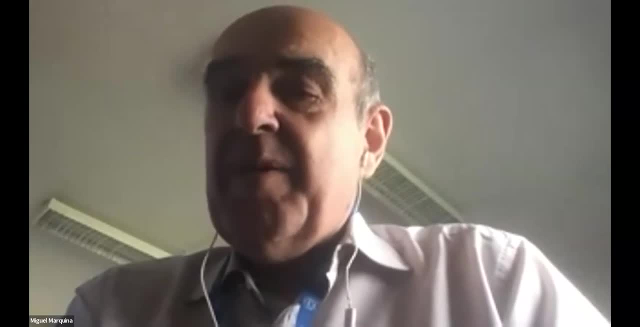 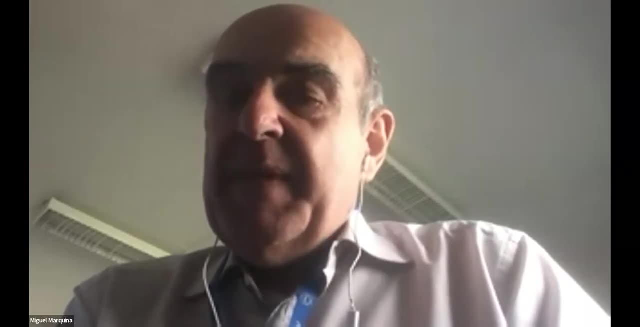 me a copy of the slides. no obligation, but if I get a copy of the slides, don't you worry, we will put it also in the same place, So you will have it available. Thank you. And then just checking with Felice. please feel comfortable at raising your questions. 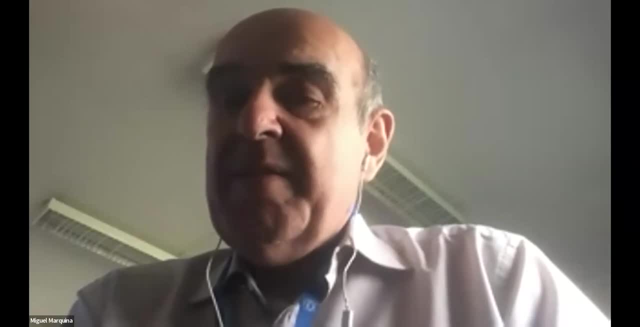 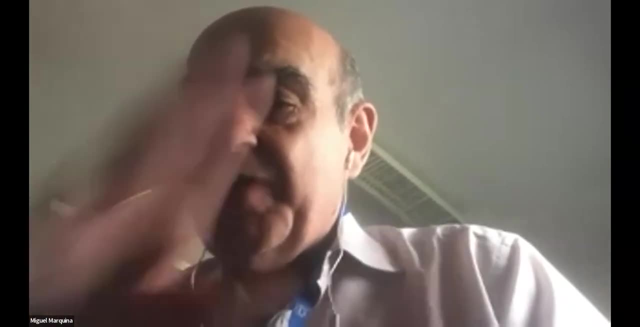 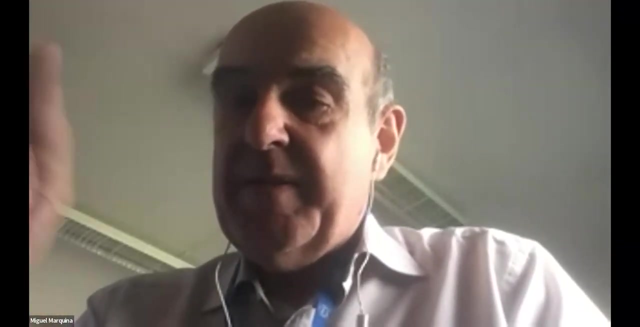 as the talk goes. Now my suggestion is, instead of raising the questions orally, to interrupt Felice. make a sign in the chat and I will keep an eye so Felice can concentrate on the talk. But if you want to have a question, I will just keep an eye on the chat and then. 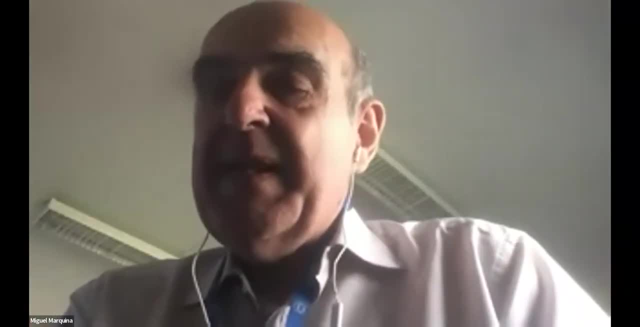 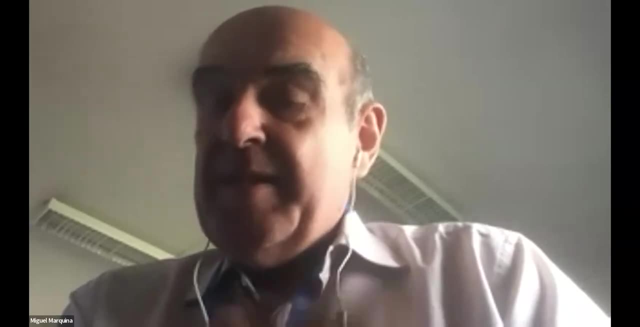 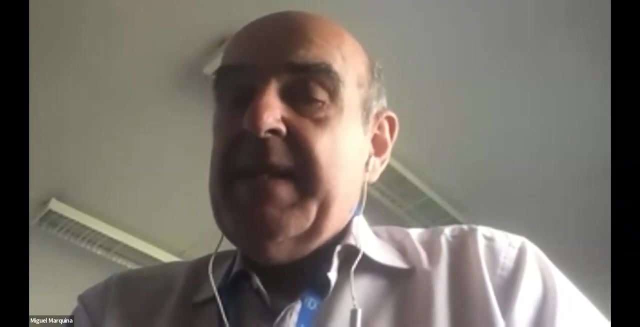 mention this to Felice when it is an appropriate moment- I don't know if in the audience- just to remind you or maybe for the first time that you hear that, if it is the first time that you're into this series of lectures, this 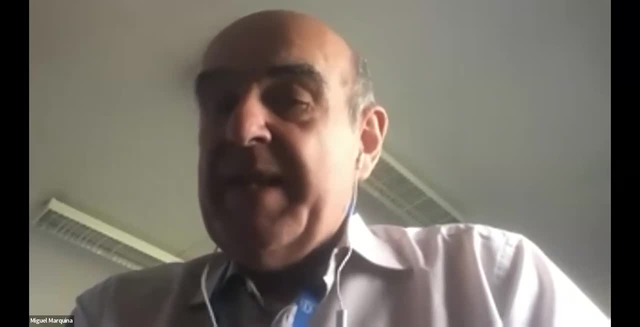 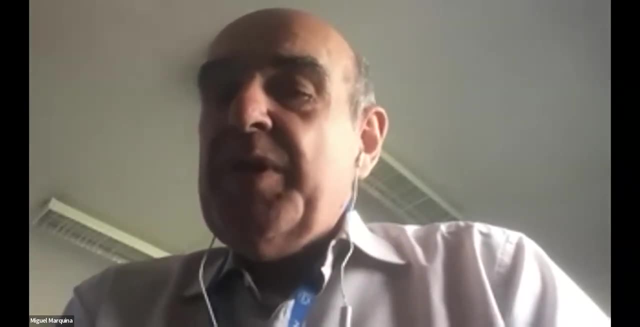 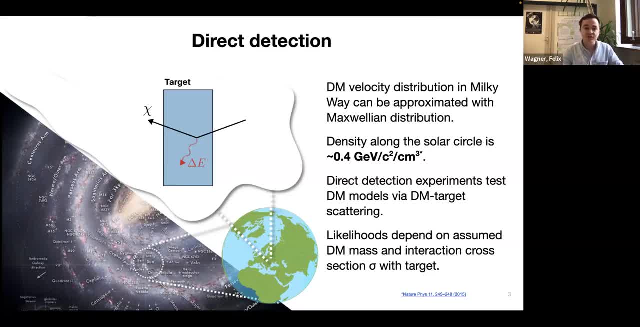 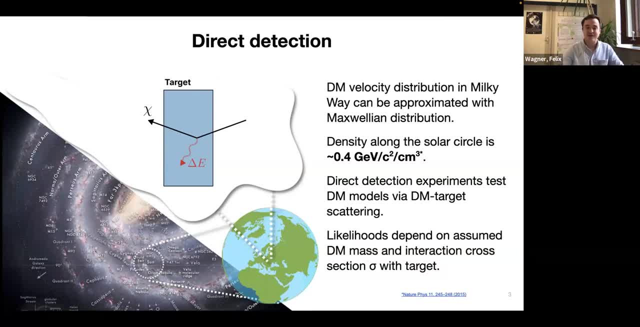 expect roughly in every cup of coffee at a point in time to have one dark matter particle. So there are quite many of them around, And if you do an experiment like that where you want to directly measure the scattering of a dark matter particle in your target, then of course the 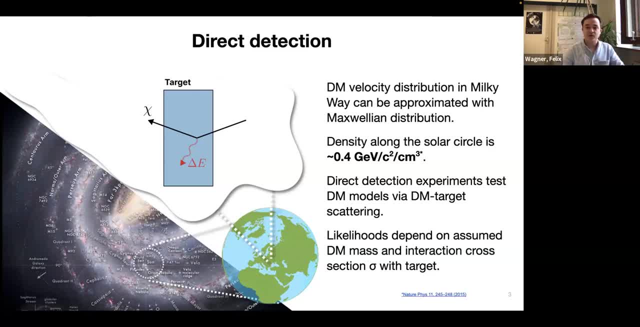 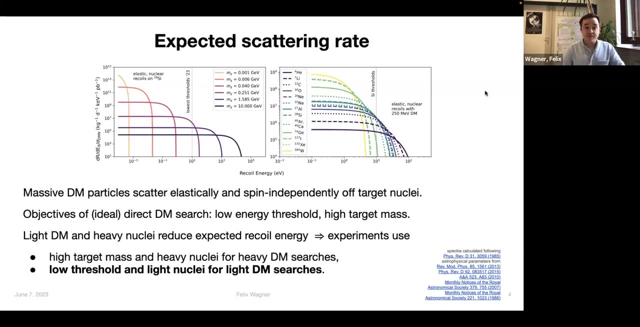 statements that you can make about the existence of dark matter depends on your assumed mass of this particle and certainly and also on the interaction cross-section of the dark metal particle with your target And if you make a few reasonable assumptions, namely that these particles would 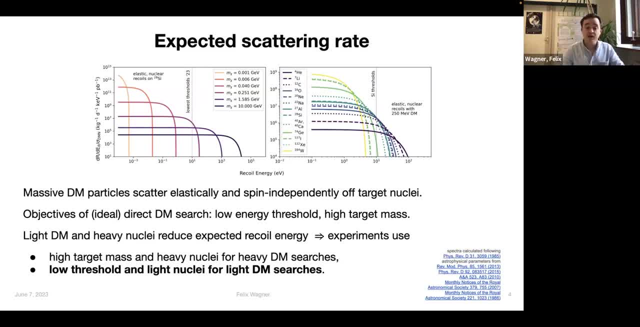 maturely scatter with your nucleus, with the nuclei in your target, and that this would be an elastic scattering, then we can calculate the expected scattering rate in the target. And to depict this I plotted here a couple of expected scattering spectra, depending on the deposited recoil energy in your target And what we can see on the left of this. 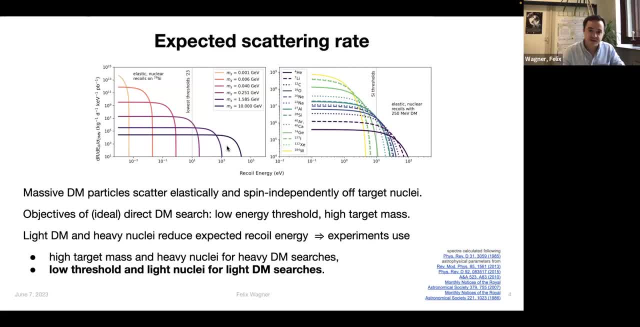 plot is that the expected recoil energy grows with the mass of your dark metal particle, or the other way around. for very light particles, you expect only very small recoil energies, And on the right side we can see that the expected recoil energy does also grow the lighter your 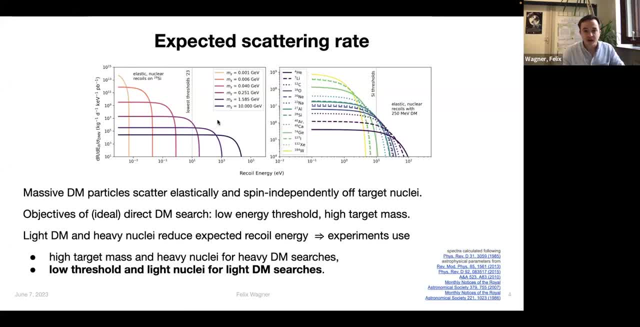 target nucleus is- And what we can see here is a straight line- the currently best achieved recoil thresholds for these direct detection experiments And therefore in practice it's easier to reach a low recoil energy threshold with a light target, so with a relatively small target. 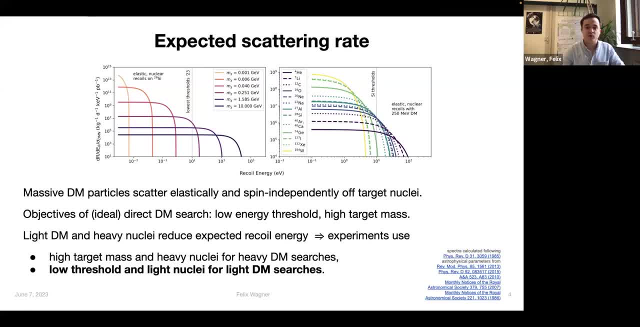 Therefore, in practice we have a trade-off, namely that the experiments that look for heavy dark metal particles or above several GeV particle mass, that they maturely use large targets to collect a large exposure and also heavy nuclei, And experiments that want to hunt these light dark 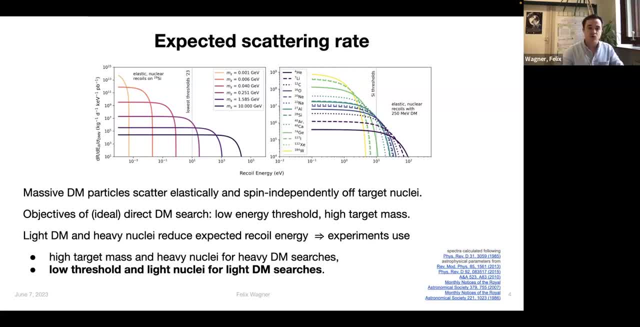 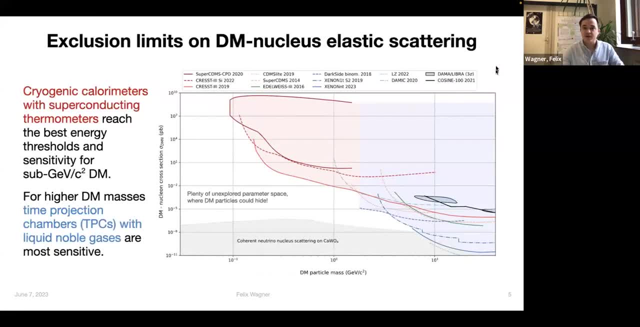 metal particles, use light targets, low energy thresholds and light nuclei for these searches And we can quantify these results from direct detection experiments in terms of exclusion limits in this parameter space. So since no conclusive dark metal signal was measured today, we can only draw these lines where we tested the 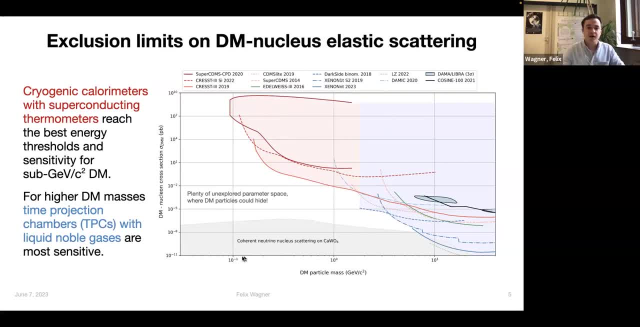 parameter space and where we can exclude the dark metal exists And this dark metal. so this parameter space is in one dimension the dark metal particle mass, and the other dimension the cross section, And we can see here two regimes where two different technologies dominate. these 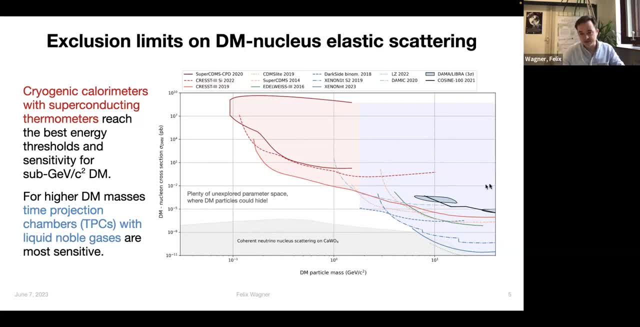 results, namely for particle masses above roughly 2 GeV time projection chambers with liquid noble gases. the mass of the dark metal particles is approximately 100M by 10G and the mass of the light metal is approximately 50G. These are different due to the different poinents of the light metal. also the dark matter particles are the light metal particles. it is a variable of light energy. The light metal masses achieve the best sensitivity, so there are experiments like Xenon or LZ or DarkSide, and for lighter masses, especially below 1G particle mass, glygenic calorimeters with superconducting thermometers reach the best sensitivity. This is mostly because they can reach these low energy thresholds that are required to measure some dark metal particle scattering in this material. 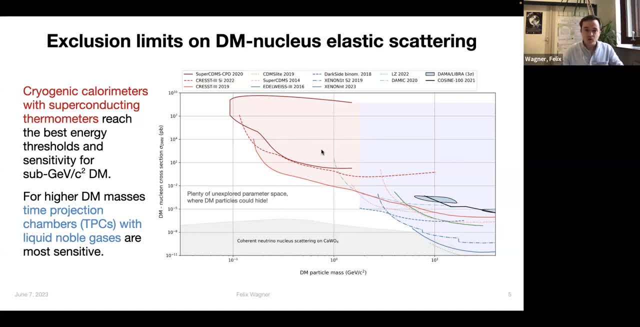 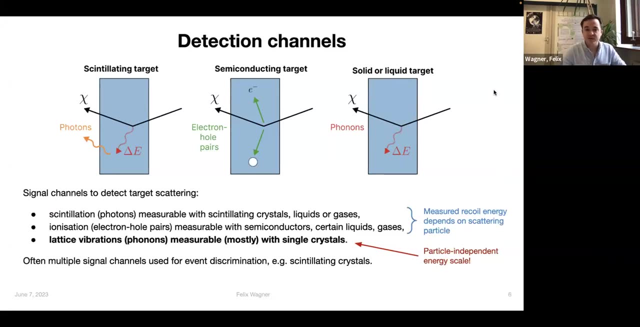 mass regime. Now to go more into the direction, how this works. so why can these experiments measure these very low energy recoils? we have to take a look at what detection channels there actually are in this type of low energy detectors, And we can here separate three. 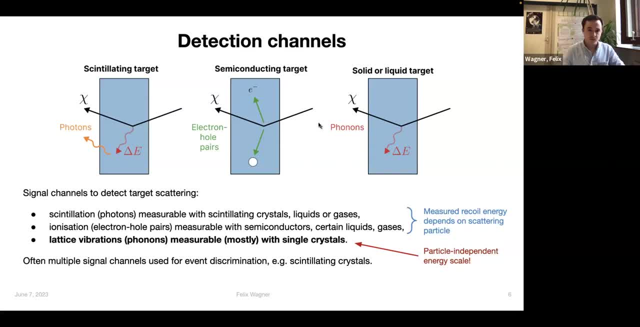 different signal channels that can be measured, namely in the particle recoil, In the particle recoil in the scintillating targets. the recoil would produce phonons that can be collected with some phonon detectors In a recoil, in a semiconducting target or in certain liquids. 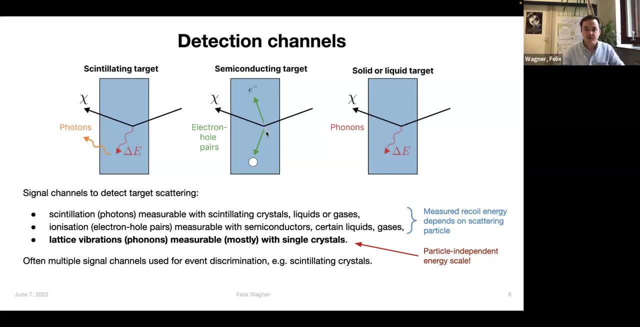 or gases, electron hole pairs are created which can also be measured. for instance, by applying a voltage and drifting these free electrons In some direction, but always in the particle scattering, you produce some vibrations in the target, in the case of a crystal, some luckiest vibrations, which we call them phonons. 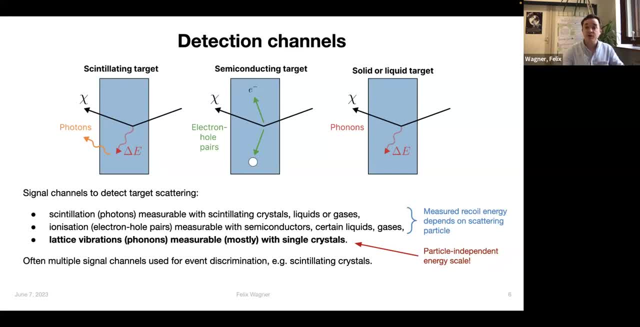 And in fact the largest share of the recoil energy is usually deposited in these phonons. So if we have a means of measuring these phonons directly, then this gives us, gives us a relative, So this gives us a good accessibility of this, of this recoil, of this deposited. 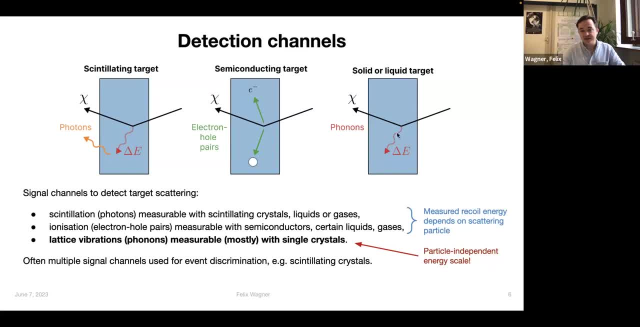 energy, And also this gives us a part of the independent energy scale, and what I mean by that is that the amount of phonons produced or the energy deposited in phonons does not strongly depend on the interaction pipe, namely if the recoil was with the nuclei of the target or with 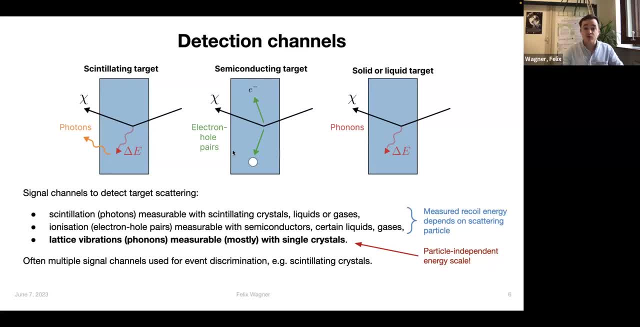 the electrons of the target in electron hole, pair creation or in scintillation. this usually depends strongly on this interaction type, And often experiments use two of the signal channels to discriminate between different types of particle recoils. But now the question is: how do we actually measure? 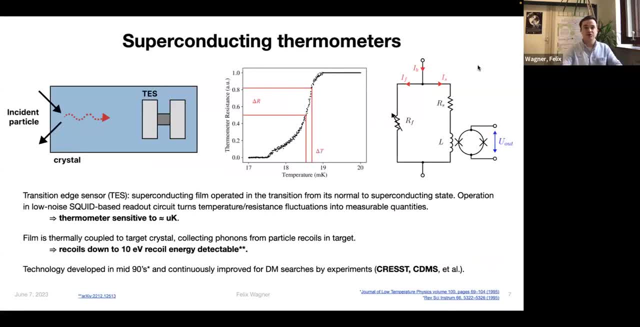 these phonons. And here our technology of superconducting thermometers comes into play. So a superconducting thermometer is a small superconducting thin film that is deposited on a target. In this case we'll talk about target crystals. So on a target crystal, And 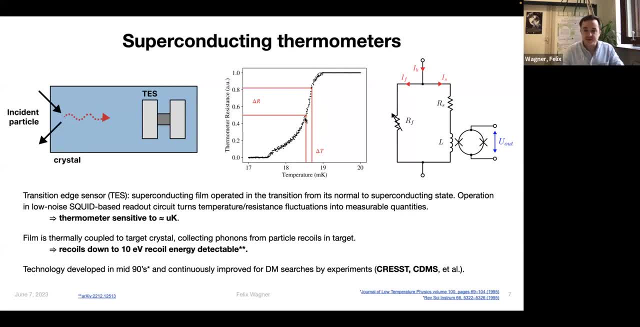 the temperature of this whole device is then fine-tuned such that the superconducting film is exactly in its transition between a superconducting and a normal conducting state, And what this means is, like you can see here in this plot in the center. 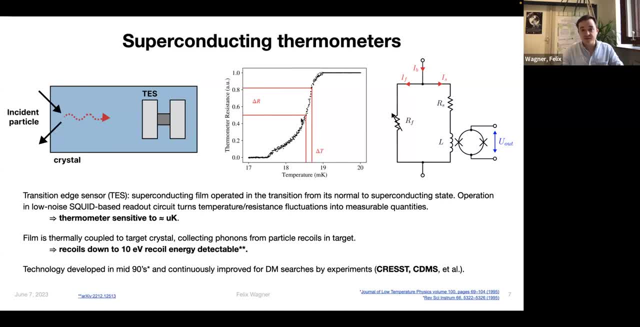 that a small temperature fluctuation causes a very large fluctuation of the resistance of this film. And here this is an example of a tungsten film. Tungsten has transition temperatures around 15 millikelvin. Here, for only a very small temperature fluctuation we would measure. 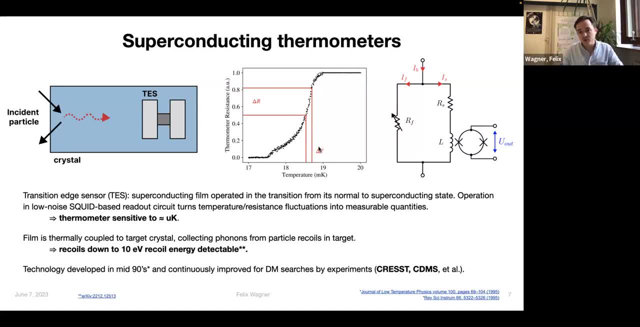 a very large resistance fluctuation. If we operate this superconducting film, then in a low noise and squid-based readout circuit we can reach with that thermometer that is sensitive to micro Kelvin temperature fluctuations. Now this thermometer: when a particle recoil happens inside this crystal, this produces. 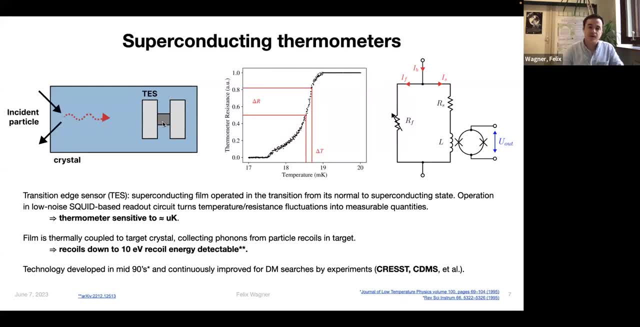 finally, some heat in the crystal, but also in the thermometer, and produces a temperature increase. And with this technology we can reach sensitivity. so we can reach recoil energies down to only 10 electron volts recoil energies. So this technology was developed in the mid-90s and since then continuously improved for dark 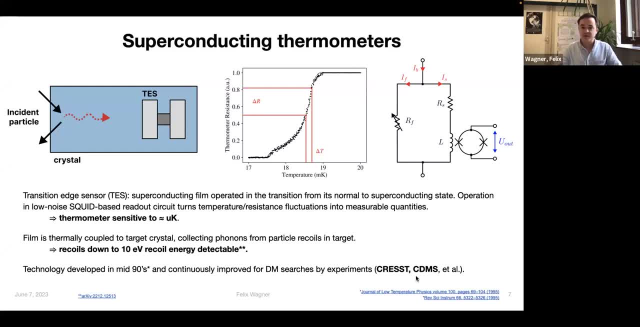 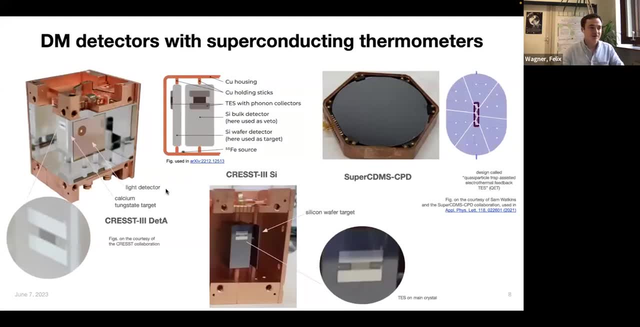 matter searches by experiments, among them most notably the CREST and the CDMS experiment, And at this point it's maybe also very nice to look at these devices how they look in the real world. So here on the left side we have a detector model from the CREST-3 experiment. 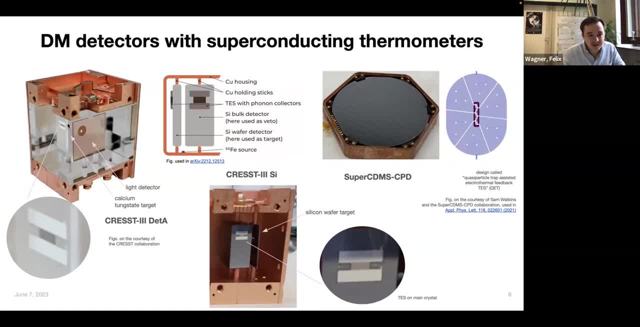 And what we can see here? this milky whitish crystal. this is a calcium tungstate target crystal And on this crystal, deposited, there is this superconducting thermometer film And down here we can see a wave. so on the side, here a wafer detector. 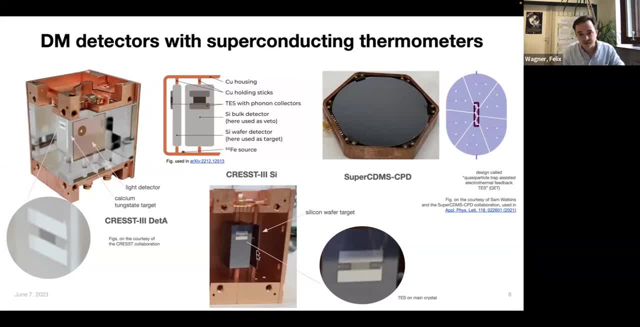 From a current run of the CREST experiment. there the target is made of silicone And you can again see this superconducting film. And on the right we can see a detector from the super CDMS CPD experiments. This is a much larger wafer. 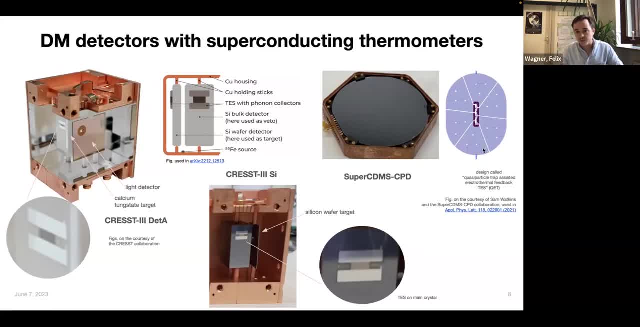 Here we can also see that the type of how these thermometers are in detail manufactured can differ. So in this case the super CDMS experiment uses here a much larger wafer. So in this case the super CDMS experiment uses here a much larger wafer. 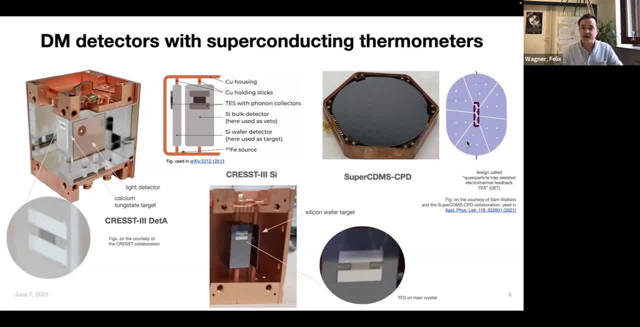 So in this case the super CDMS experiment uses here a much larger wafer area of aluminum phonon collectors, and in just a bit we'll talk more about this type of collectors. Okay, with that, let's look a bit more into the details of the physics that happens here in the 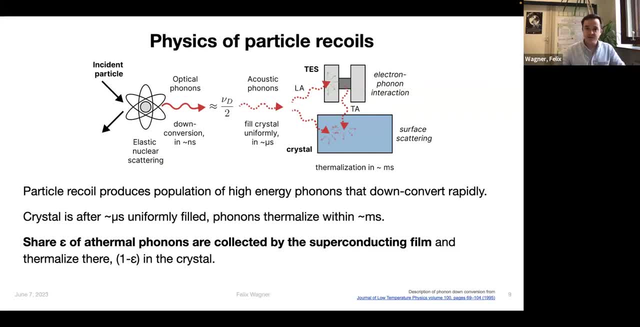 sensor. When a particle recoil happens in this crystal, the particle recoils, so we assume that this particle recoils with the nucleus in the target and this produces a large population of high energy phonons, namely, in this case, optical phonons. Optical phonons are a phonon mode with 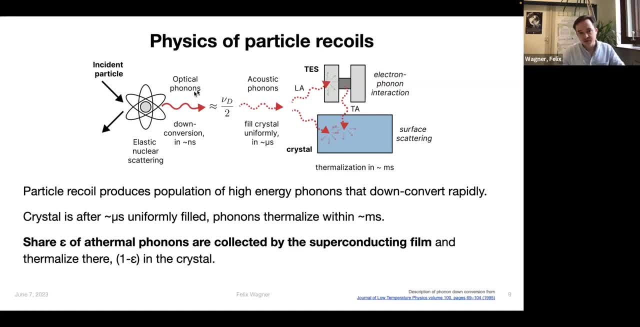 much higher energy. but these optical phonons, they don't travel very far in this crystal so they exist only relatively, so localized around the position of the recoil, because they down, convert in the lower energy phonons Very fast, namely on the time scale of nanoseconds, and with up after this initial 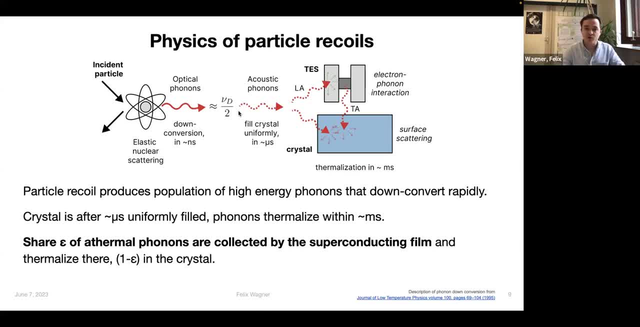 down conversion. you end up with a large population of acoustic phonons of about an energy of about half the bifrequency in this material and within several microseconds. these acoustic phonons fill the whole target crystal uniformly and then they thermalize, so they down convert further to thermal. 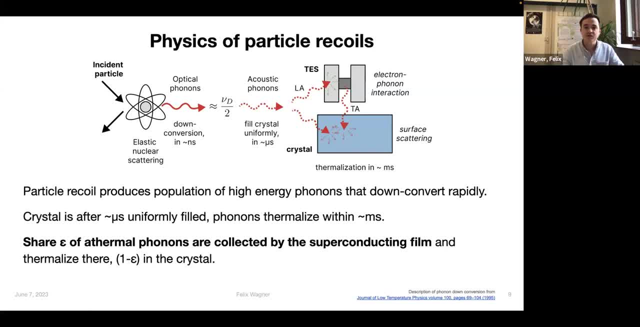 For phonons, of which we can then think as just heat, and they thermalize mostly due to processes, namely the electron phonon interaction in this superconducting film and surface scattering in the crystal. and now it depends on the how this device is in detail manufactured, which share of 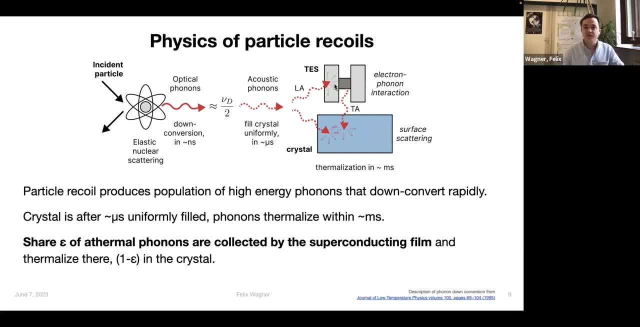 this initially deposited energy thermalizes in the superconducting film, so in the thermometer, and which share thermalizes in the crystal, And we call this share, the parameter, epsilon. so share epsilon of this recoil energy ends up as heat in the superconductor and the remainder, the 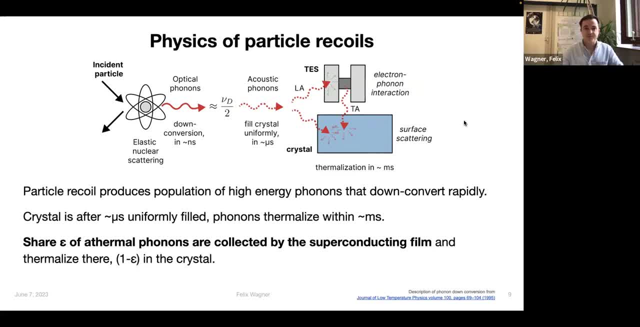 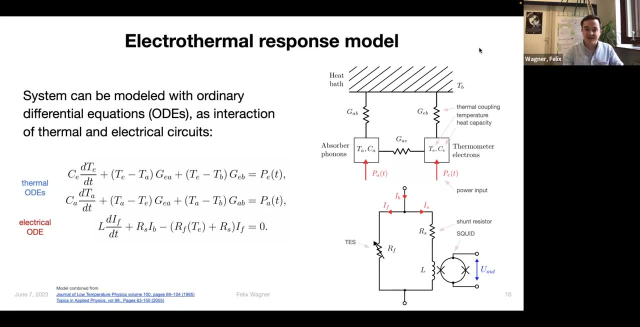 share, one minus epsilon, ends up as heat in the crystal. And if we take all this and put it together with some standard methods from electrical engineering, we can in fact derive a system of differential equations that mathematically describes the sensor type. To do this we consider the two, the two main, so the two dominating heat capacities in the system. 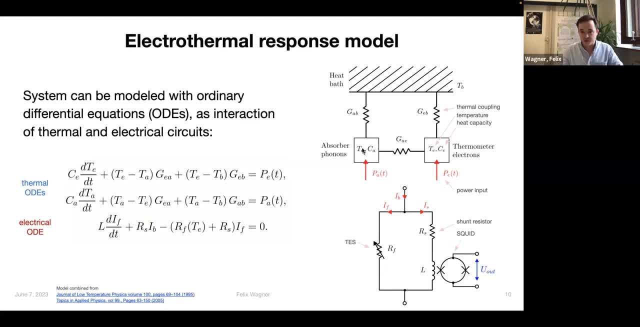 namely the photonic system of the crystal, which is a non-metal, and the electronic system of the thermometer film, and we connect them with heat capacities and so with thermal couplings, and connect them also to heat, And this we can then put with the heat equation. we can put this into a kind of collapsed heat. 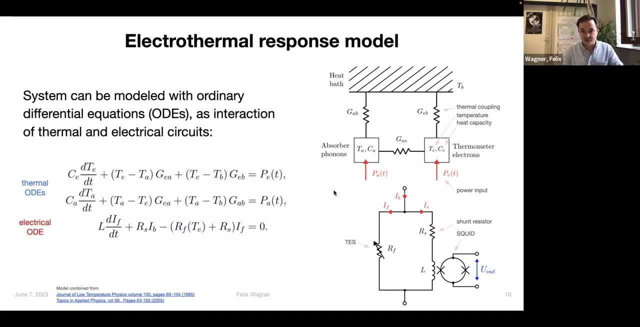 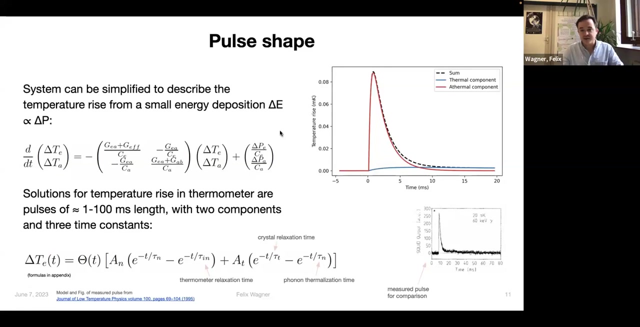 equation. we can put this into a system of differential equations and we can in this system also include the electrical differential equation that describes this readout circuit and with that we can already do some calculations of the expected detector response for such a device And In fact this expected response for a small energy deposition, like we expected from a low energy. 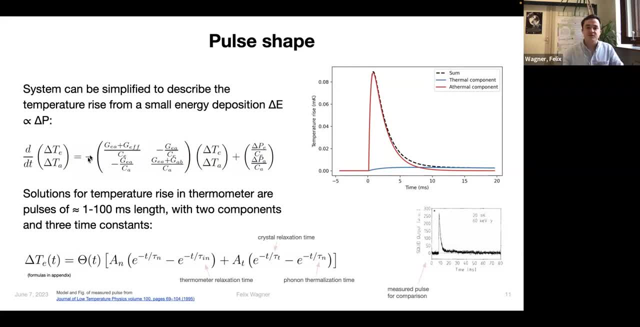 particle scattering or light stark matter. So this, we can simplify this system and solve it analytically, and we end up with an equation that has three major parameters, namely three time constants, out of which one is the thermalization time, the effective thermalization time of these phonons. 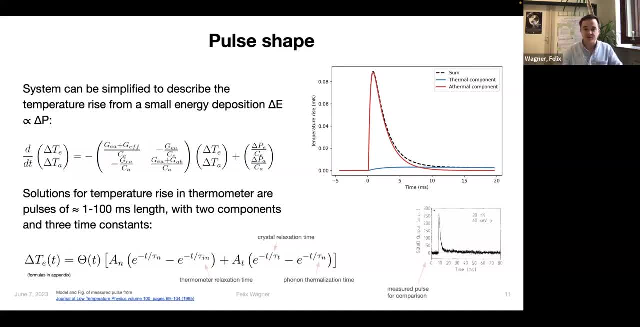 One is the thermal relaxation time of the thermal relaxation time of the phonons, One is the thermal relaxation time of our superconducting film And the third one is the thermal relaxation time of the crystal. And, as you can see here in this equation is that two large components appear in the solution. 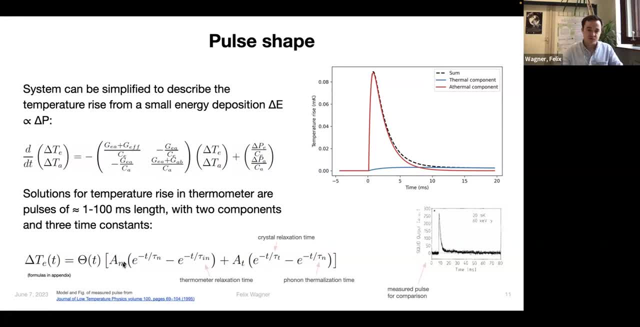 out of which one is caused by the thermalization of the phonons in the superconducting film And the other is caused by the thermalization of the phonons in the crystal. and if we fill in some meaningful values for all these parameters and plot this detector response, we can see that the 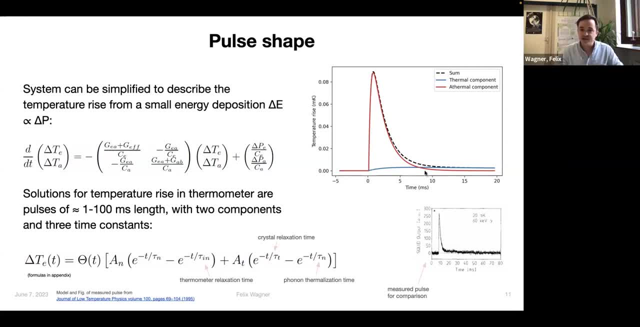 measured detector response from such a particle recoil is a two component pulse where for typical devices, this first component, which comes from the, the thermalization of the art, thermal phonons in the, in the superconductor directly, is the dominating component. That also, that also gives us the sensitivity of this device. 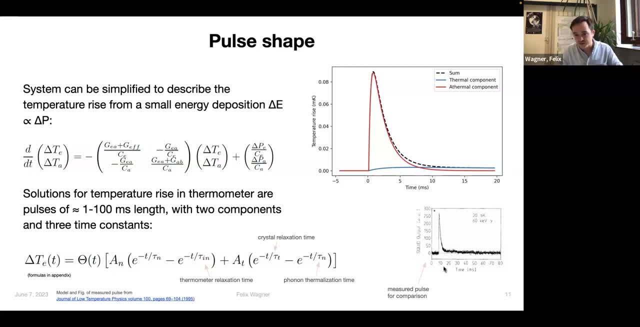 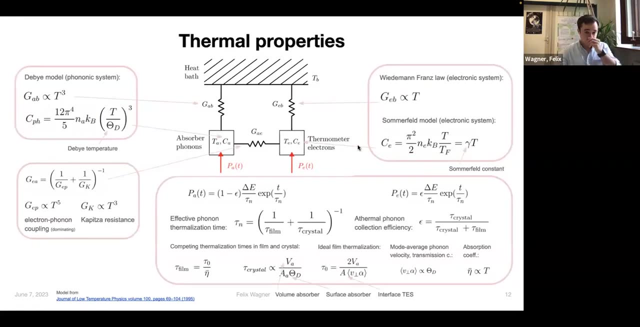 Yeah, and for comparison, to show you how these pulses really look like when you measure them, this is from the paper where I used these parameters from a pulse that was measured Okay, and now one could in fact say now a lot about how to calculate all these physical parameters. 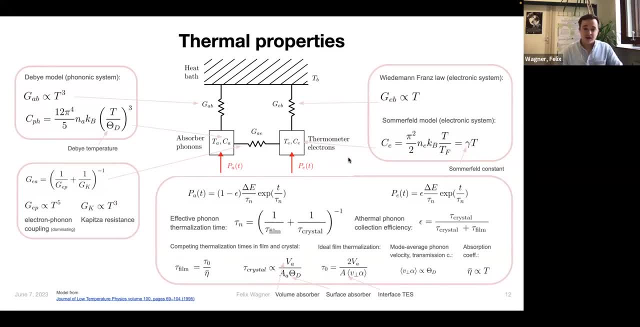 But I don't want to go into that much of a detail. rather later on we'll look at some practical scaling laws. so maybe what we can take away from this slide here is that this: we assume that this thermalization of the phonons happens on an exponential time scale. This is equivalent. 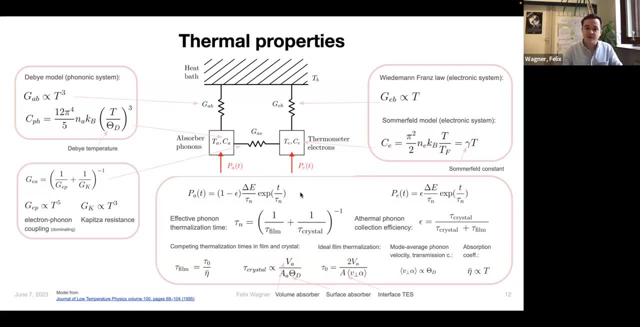 to saying that we assume that there is a monochromatic phonon distribution in the crystal, which is probably not exactly the same- There is probably some​- this case in reality- but which is a practically in practice a very good approximation- and that all of these thermal couplings and heat capacities are either dominated by a photonic system or 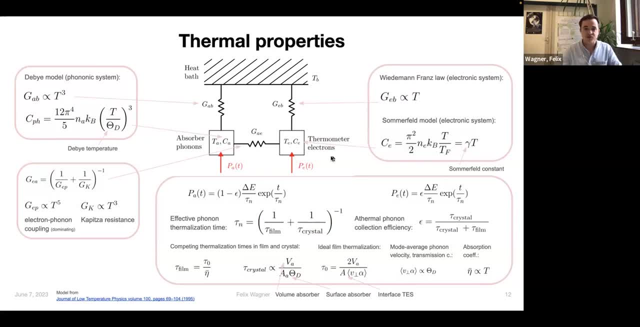 electronic system and there are some models to reliably calculate them. so especially these heat capacities can be calculated quite reliably. for the thermal couplings. they depend a lot on the details of how this device is manufactured. so in practice one usually takes some measured values from similar devices if one wants to estimate some sensitivity of a new device. 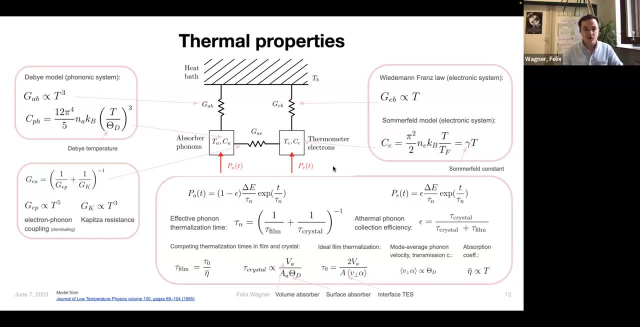 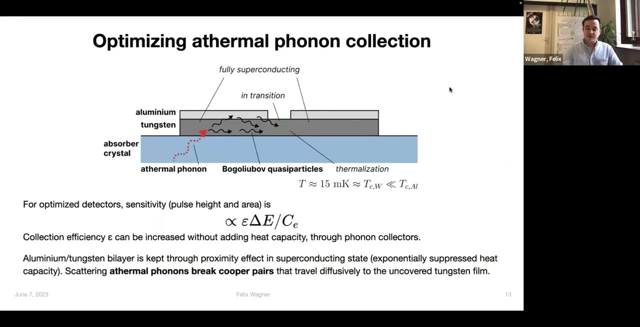 and all of these quantities depend strongly on the temperature of operation. okay, with that, let's look a bit into the sensitivity of these devices. so what are the crucial quantities that determine the sensitivity of this superconducting thermometer type detector and, as we saw before that, the 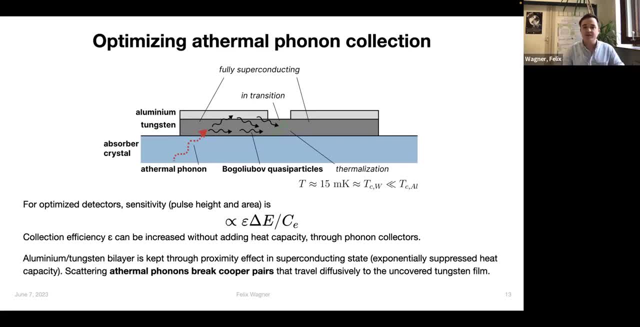 atemal part of the pulse shape, namely the temperature increase that is produced by phonons that thermalize directly in the superconducting film, is the major factor that determines the sensitivity and we can approximate in an optimized device. we can approximate this atemal pulse shape with the 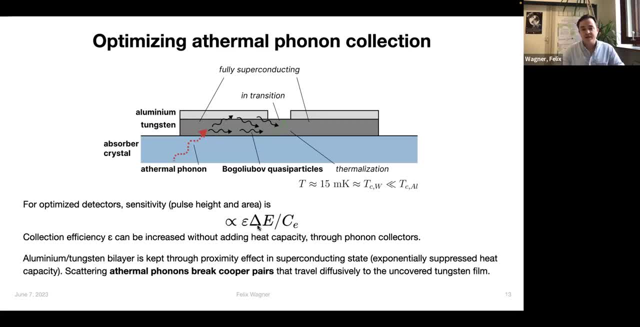 correction efficiency. so this parameter epsilon and the deposited energy in the particle recoil, but then the heat capacity of this superconducting film. so it's inversely proportionate, the heat capacity in the superconducting film, which kind of makes sense if this is a larger. 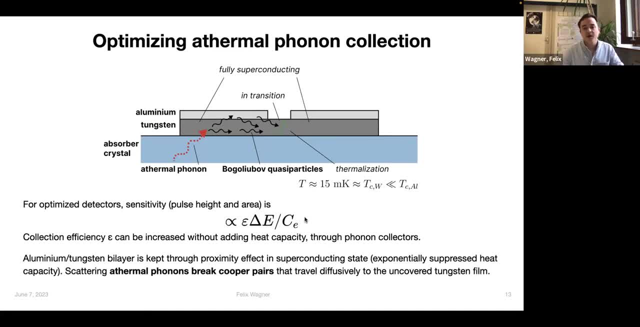 piece of film, then you need more energy to heat it up, and there is one technology that was kind of a game changer in the past couple of years, decades, to significantly amplify this collection efficiency and, with that, the sensitivity of the device. this is called a phonon collector. they have it depicted up here. so what we see? 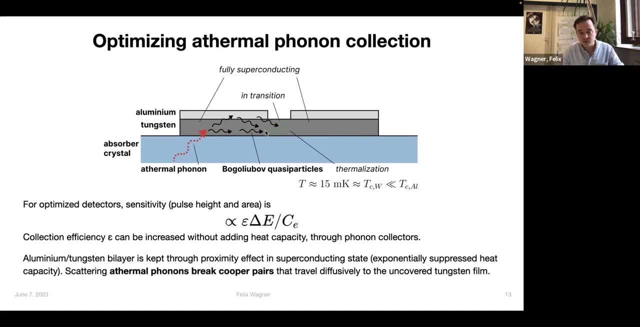 here is this tungsten layer which we use as the superconducting thermometer. we operate the whole device in a within the transition of the tungsten, but then we cover a large area of this tungsten, aluminum, and aluminum has a much higher transition temperature, so at the operation temperature this 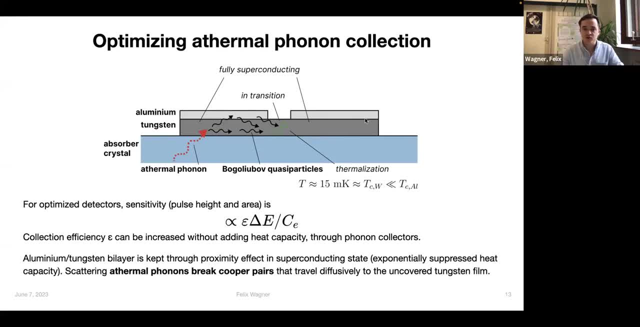 aluminum film is already fully superconducting and due to the so-called proximity effect, the tungsten that is covered here by aluminum is also pulled into a superconducting state. Now the heat capacity of a superconductor or the heat capacity of a metal in its superconducting 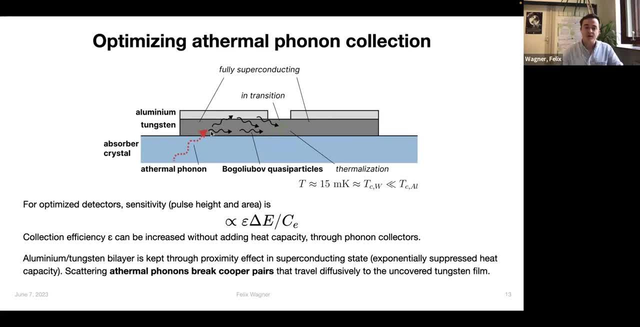 state is suppressed exponentially compared to its normal conducting state and therefore, what happens when this so? therefore, this does not significantly. this tank, this aluminum covered tungsten part, does not significantly contribute to the total heat capacity of the thermometer. But what happens if we have this r-thermal, this high energy phonons scattering in this? 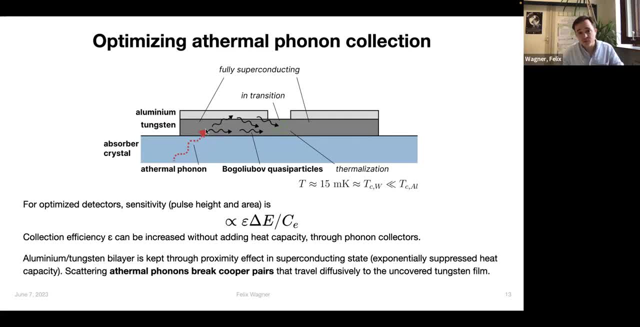 superconducting film is that you break. we break copper pairs here, and these broken copper pairs are also called bogor-yubov quasiparticles and they travel diffusively in the superconducting film until at some point they reach this uncovered tungsten film which is in transition and deposit their energy there. So by that we can kind of 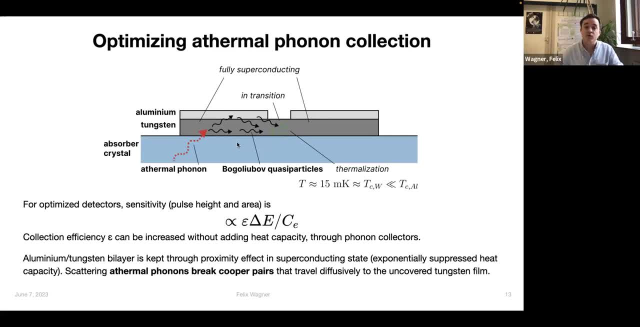 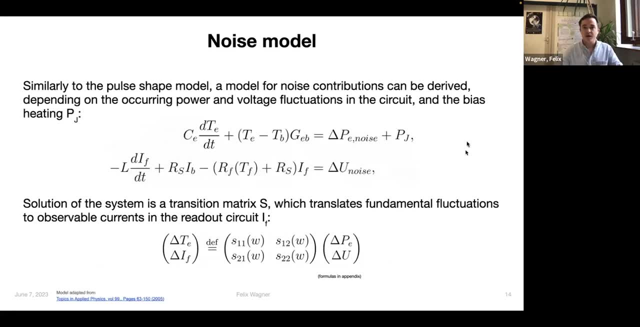 increase the amount of collected r-thermal phonons in our sensor without increasing the heat capacity. Now, talking about the sensitivity of such devices, we already need to think. we not only need to think about the strength of reaction or to particle recoils, but we also need to compare this with. 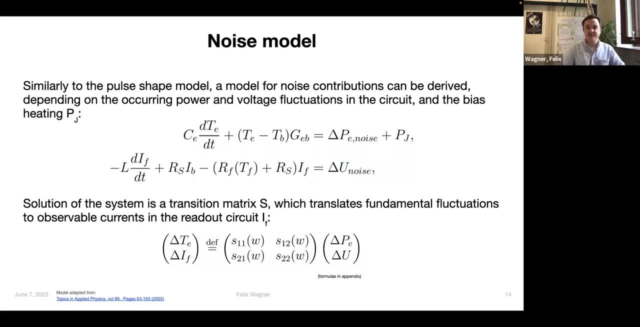 the omnipresent sensor noise in these devices and for that there are also models to predict this noise. namely, we take again our our system of the differential equations that we established a few slides before, and if we solve the system for small fluctuations of power and voltage in the radar circuit, 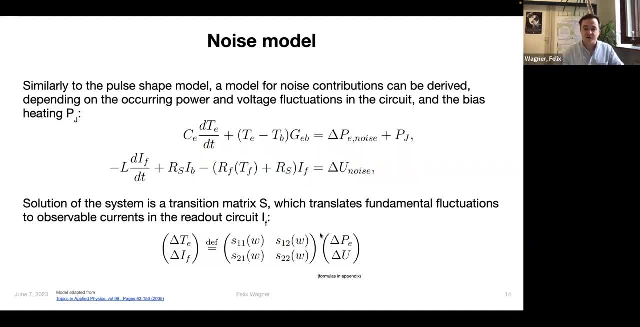 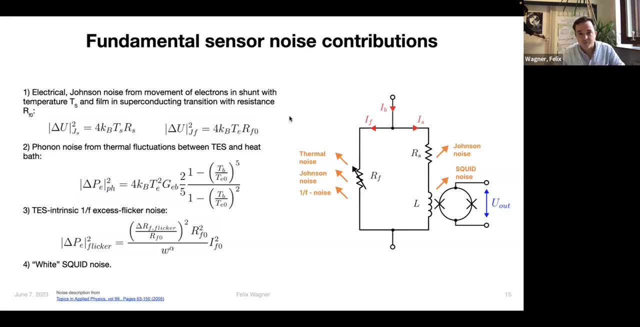 if we solve the system in foyer space, we can derive a kind of transition matrix that gives us the expected noise fluctuations from fundamental power and voltage fluctuations in our system. and there are mainly four well studied and well understood sources of noise in these devices, namely the electrical johnson noise which appears in each resistor in this readout circuit. 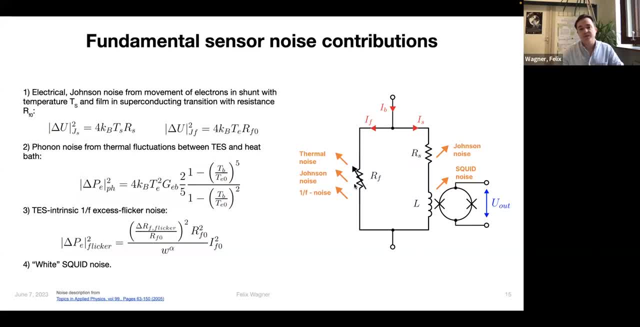 then the thermal, also called phonon noise, that happens in the in the thermal coupling between the ps and the heat path. then the white or frequency independent squid noise which is decoupled from the heat path, from this reader circuit, and one prominent noise source is the so-called excess one over f noise. 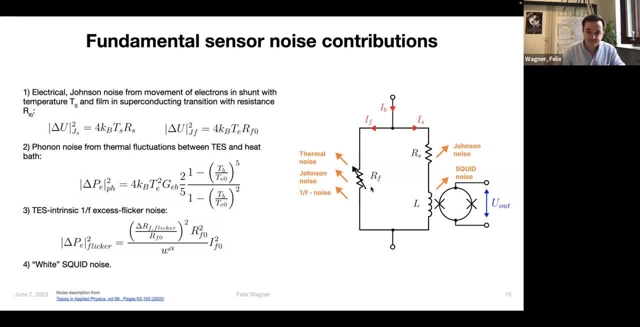 this is a intrinsic excess in the superconducting film that is probably caused by the some fundamental fundamental properties of superconductivity, but it is not very well understood until today. so this is not reliably reliably predictable but has to be extracted from measurements. and in fact this is not the only excess noise source that appears in this type of devices. 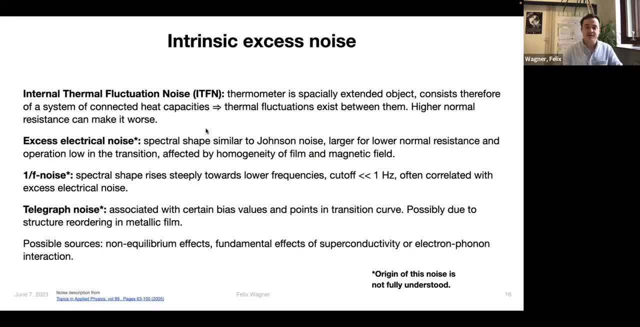 but there are several intrinsic excess noises that can only be realistically described with the, with the current models. one of them is internal thermal fluctuation noise. this is a kind of well understood noise source, and this just comes from the fact that, in reality, this superconducting film 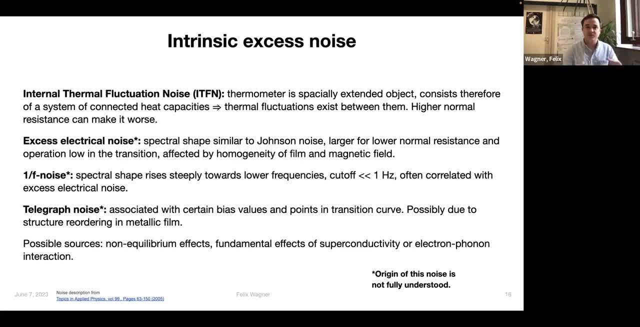 is not collapsed to one point in space, but it is a spatially extended object and therefore consists of many small heat capacities that are with each other thermally coupled. but there are also a series of noise sources that are where the fundamental origin is not very well understood yet. so there is observed some excess electrical noise, then- this already mentioned- one over f noise. 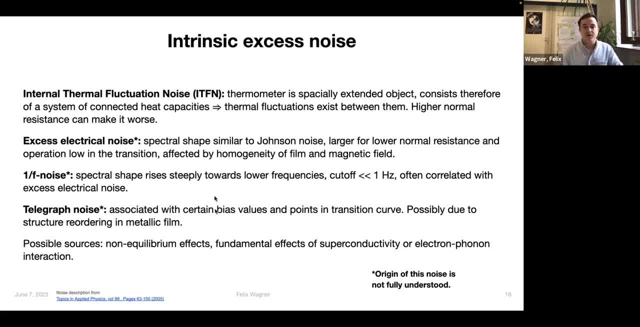 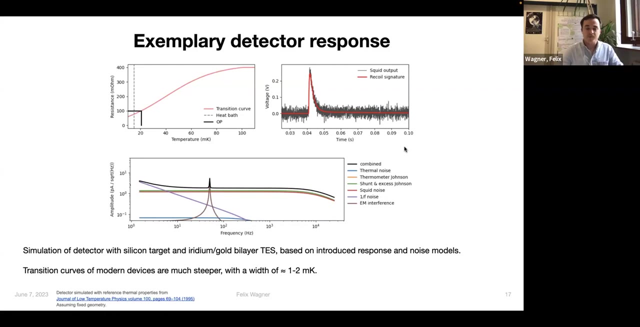 and also type of telegraph or jump noise and possibly this. so possible sources for this noise are some, either non-equilibrium effects or some fundamental effects of superconductivity or the electron phonon interaction. so, however, putting all of this together, we can based on some, if we 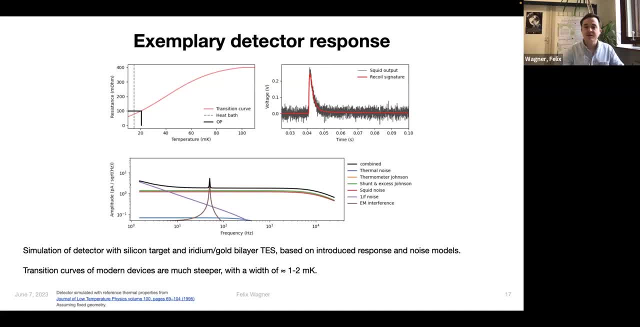 if we take the data from some measurements, we can build a simulation of such a detector, and for this lecture i did this to give a few more practical examples how this, how these devices look like if you build them and operate them. so i used from this original. 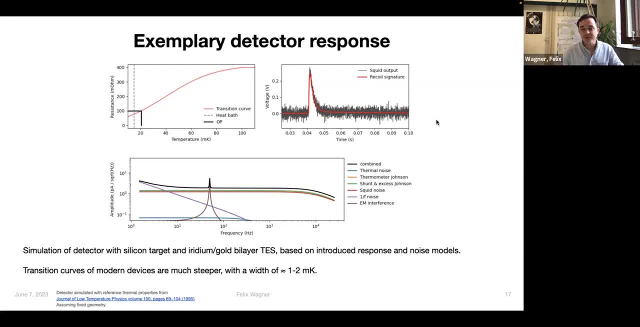 reference of the of the model, i used the static heat capacities and thermal couplings. if you combine this with the models, then you can simulate such pulses as the would appear in the real experiment. this is what you see here on the right upper plot, and here i've plotted the approximation of the superconducting transition curve. 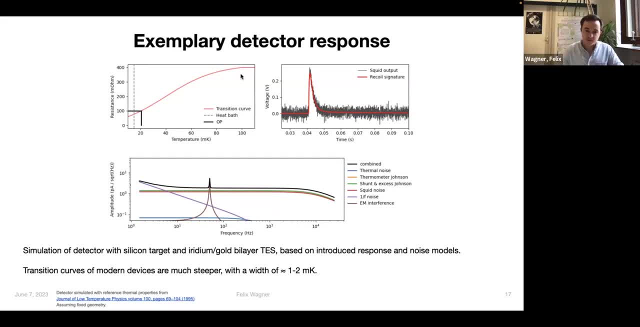 here. it is to note that for this reference, the was used, the iridium gold b layer tds, which has a very wide transition curve, namely from some some temperature slightly above 100 millikelvin down to down to 20 millikelvin and below in modern devices that are optimized for sensitivity. 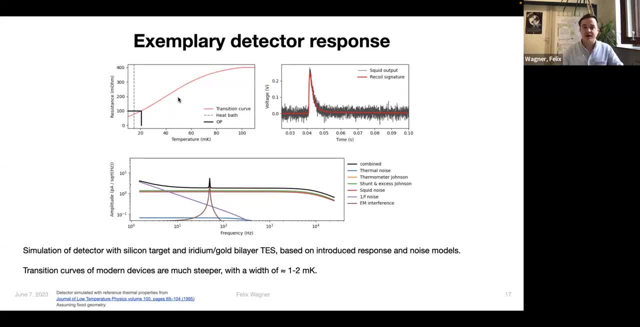 we would usually you very often i use tungsten tss which have a much steeper transition, namely with a width of only one or two millikelvin, and then down here we can see these noise sources plotted, so the noise power spectra with its components, and we can see that. so this is. 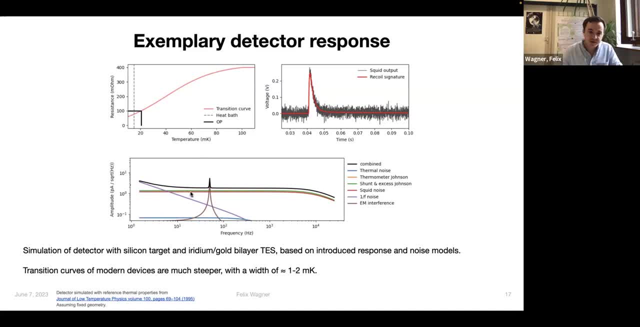 very often observed similarly to this, that for frequencies above several hundred hertz this electrical noise dominates the noise power spectrum, but for lower frequencies this excess 1 over f noise dominates the frequencies. i have here also plotted the noise contribution of a 50 hertz power supply. 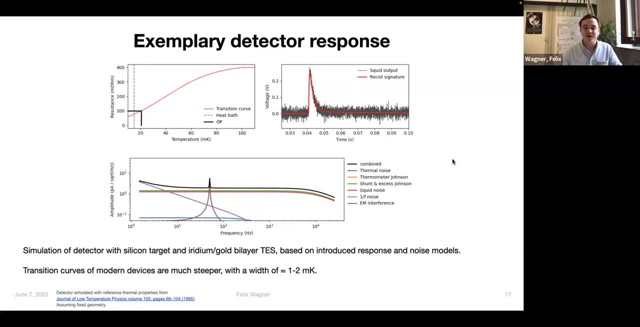 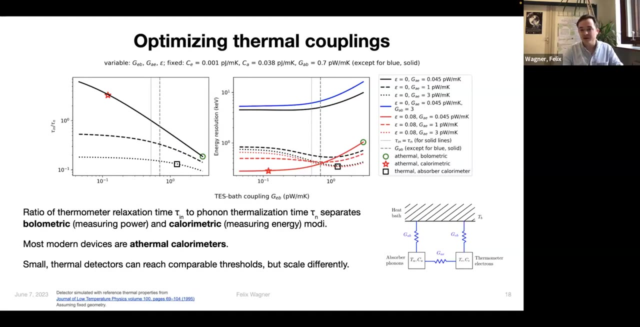 which is something that we typically also see- the noise power spectrum of such measurements. and now, having established this kind of theory, we can look at some, we can play a bit with these parameters and reason about what would happen if you would make some small changes in the, to the, to the 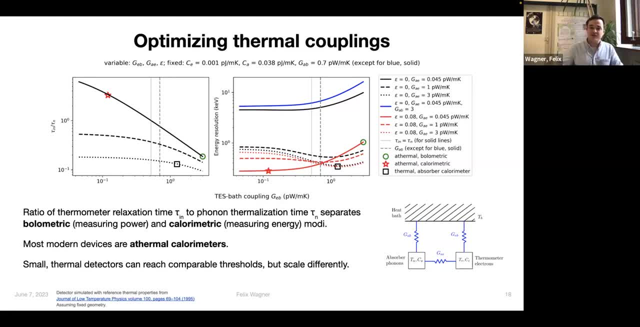 physics of this model, and with that i want to start with. so i put here this again, this thermal model of our detector again, and i want to start playing around with these thermal couplings between the heat bath and our superconducting film and the crystal and want to ask the question: what happens in this device if we increase or decrease the strength? 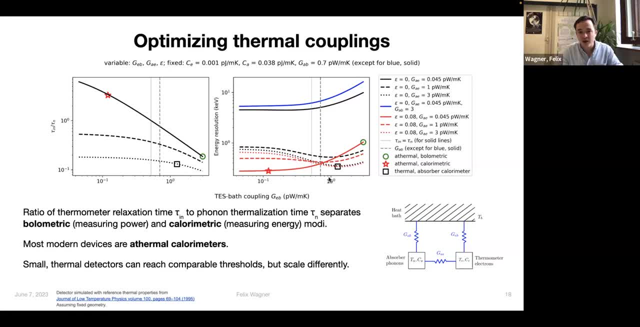 of one of these thermal couplings, and so this plot is probably something that one needs to look at twice or digest a bit, but i will guide you through it. so what we see here is red solid line. this is kind of the device that was originally used in in the reference. 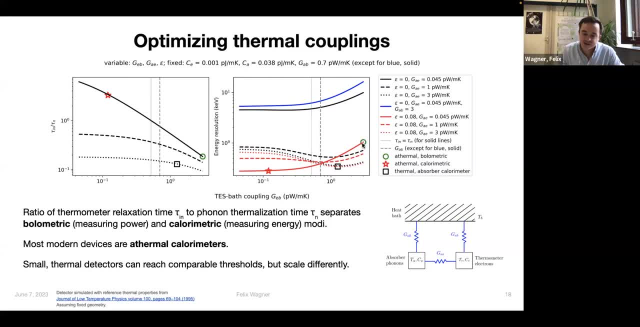 and this green circle marks the points marks exactly this detector from the reference. what we have on the x-axis is the thermal coupling between our superconducting film and the heat bath. this is typically realized by some small. this is typically shunted by some small gold film or 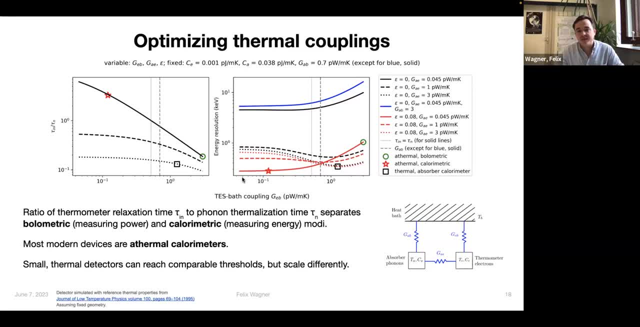 gold wire and we can, by the density of this film or the other length of this wire, we can kind of control strength of this thermal coupling. and we can see that in this original reference the detector was in a type of it's called a polometric mode, and what this means is 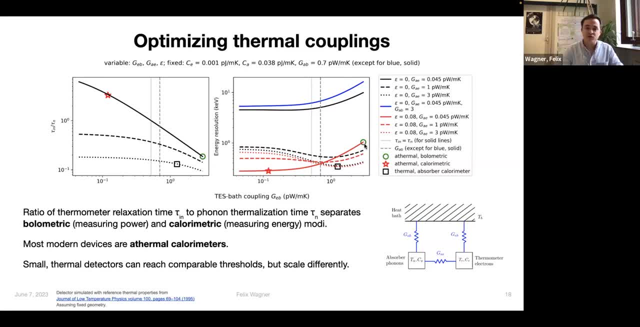 that the thermal relaxation time of the superconducting film, that this is smaller than the thermal relaxation time of the phonons, uh, so it kind of measures the power that comes in instead of measuring the total energy that is deposited. and by by lowering this strength of thermal coupling of the superconducting film to the heat path, 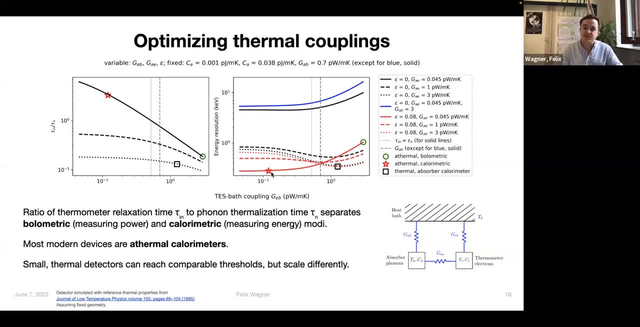 we also increase the thermal relaxation time of this film until we reach a regime which we call calorimetric mode, where the film kind of collects all the energy of the incoming thermalizing phonons before it starts releasing this energy back into the heat path. This is called the calorimetric mode and most modern devices are operated in this. 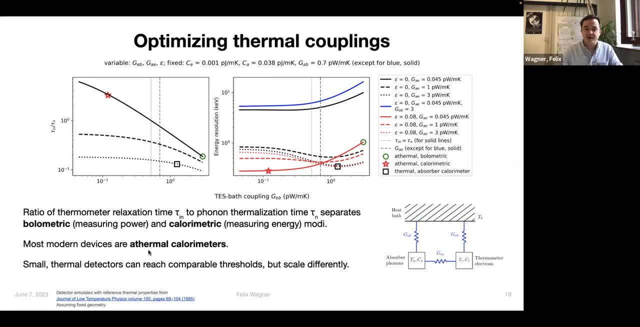 calorimetric mode, So one could say that most modern devices are athermal calorimeters. There are a couple of more interesting things that one can think about in this plot. Namely, there are also devices that are optimized to collect this thermal component of the pulse. 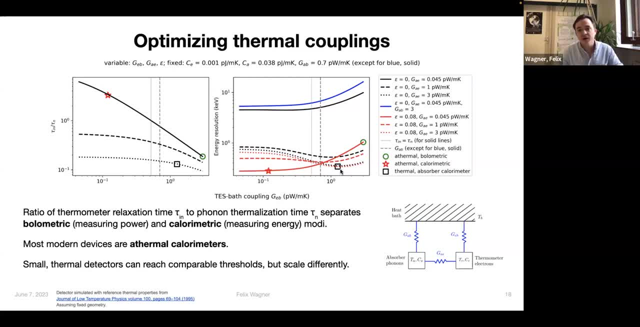 so the second pulsed component, And for small devices, this can in fact reach similar sensitivity than the athermal detectors, as we can see here. This would be the point with the black square on this plot. here, Of course, you have to optimize this device differently. So, for instance, you need a very strong connection. 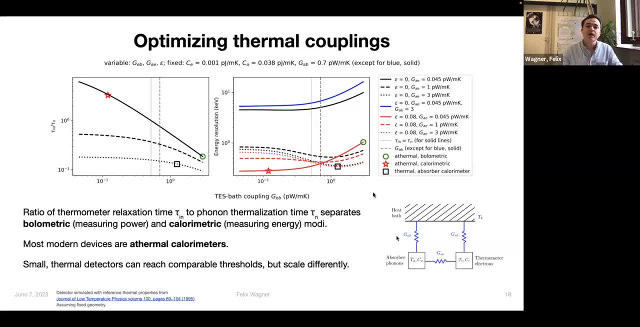 between this photonic system and the electronic system. But these devices would scale very differently because the sensitivity of such devices would scale with the heat capacity of the crystal, which especially scales very strongly with temperature, and also with the size of the crystal and not with the capability of collecting. 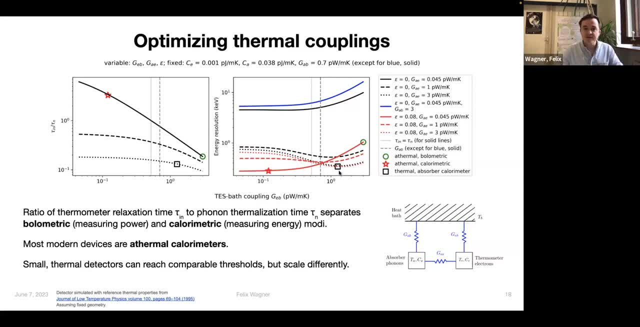 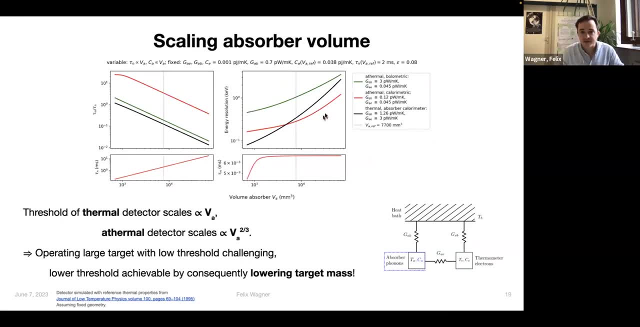 athermal photons from this crystal And to make this a bit more clear how this scaling would happen, I have here a second plot where I compare exactly these three regimes. So this original athermal bolometric mode for this detector from this reference, then the adaption to a athermal 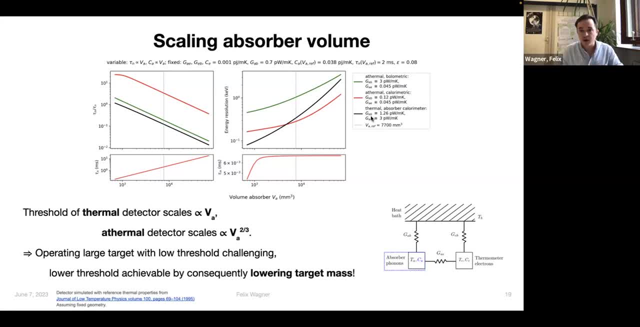 calorimetric mode. this is the red line here and the black line, which would be an optimized thermal detector. Now we want to look at this absorber and of course it would be beneficial to have the target large to collect a larger exposure. but the question that we want to ask now is: 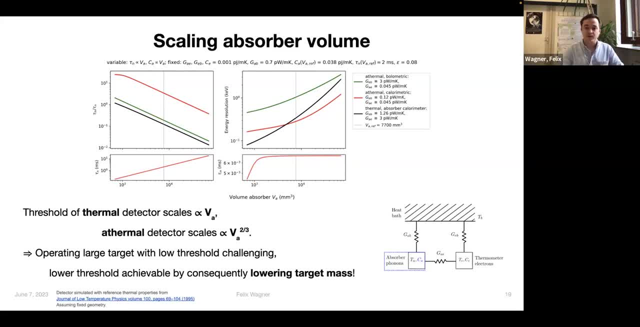 what impact has this on your recoil energy threshold, so on the sensitivity of your device? And this is plotted in the right upper plot here. Namely, we can see that for this thermal detector, the energy resolution which is proportional to our energy threshold scales very strongly with the size of our target. 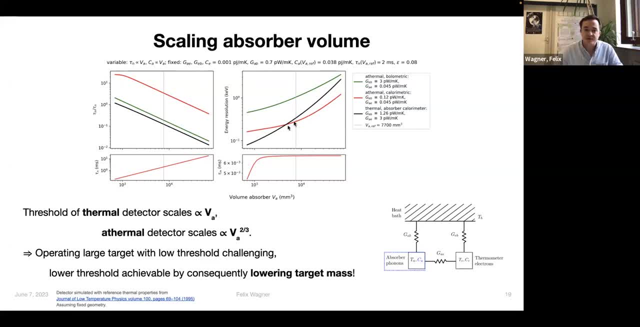 Namely approximately with the volume of the target, While the energy resolution scales not as strongly in R-Thermal devices optimized for R-Thermal phonon collection. So this is one of the reasons why current devices are mostly operated in an R-Thermal regime. 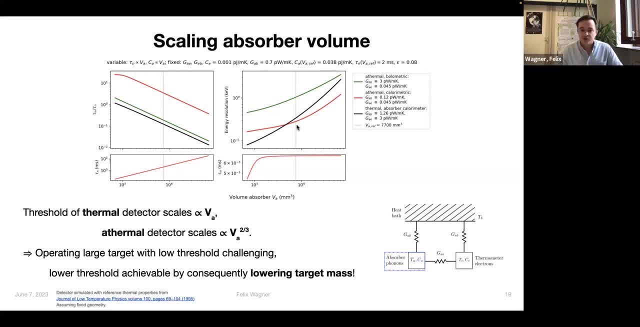 because you can scale up this target at least a bit and still reach a relatively low energy threshold. But also, what we can see on this plot is to really reach the lowest energy resolutions and thresholds, which is the ultimate goal of a light dark matter search. 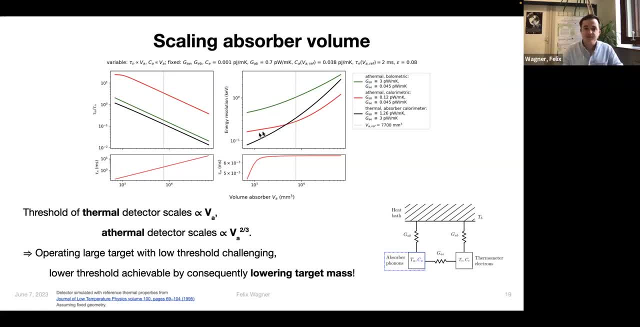 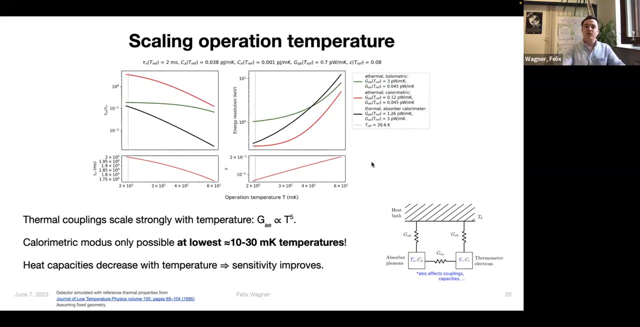 We need to just lower this target mass And this is what is also done in experiments. So current devices are relatively small targets that reach low thresholds And now we can also see- I also asked the question I always talked about- now- this very low transition. 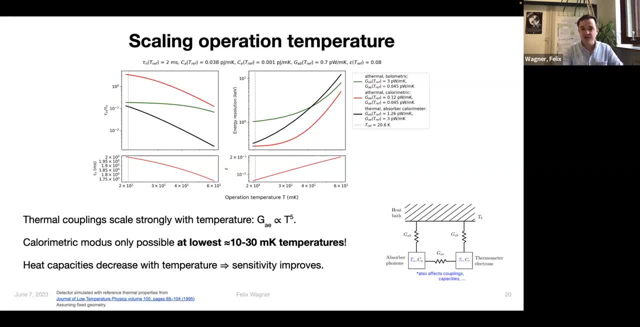 So these devices with these very low transition temperatures? So is this really necessary? operating a cryostat at 50 millikelvin or the base temperature of 10 millikelvin or lower, It's of course much, more, much more difficult than operating a cryostat with some 4 kelvin or so. 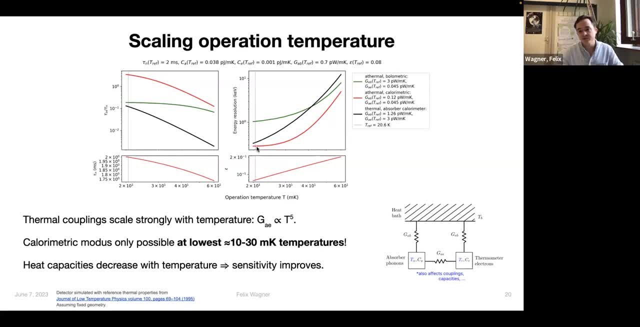 So we can ask the questions: what would happen if we lose the device with just a just a hotter operation temperature? And what we can see here if we scale up this temperature, and in this case only from the nominal value of 20 millikelvin up to 60 millikelvin? 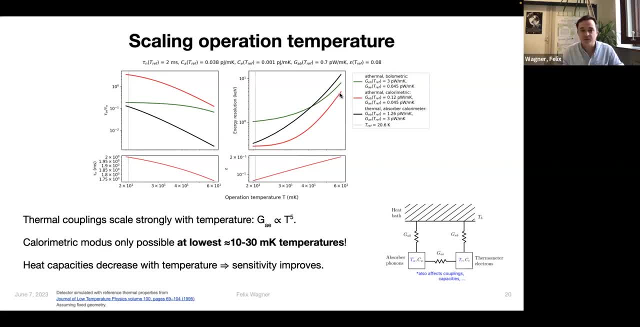 we can see a dramatic increase of these energy thresholds, therefore a dramatic loss of sensitivity, And this is mostly due to two reasons, namely that this coupling between the the electronic and the photonic system, which has to be very small for to reach an athermal calorimetric mode, 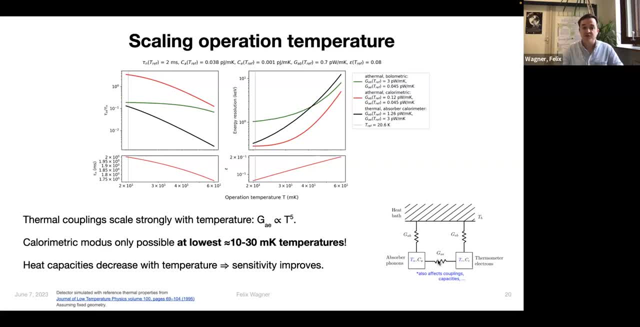 This coupling scales extremely strongly with the temperature. So this is the strength of the electron-phonon interaction that dominates this coupling, And this scales with temperature to the power of five. So this calorimetric mode can really only be reached in this. 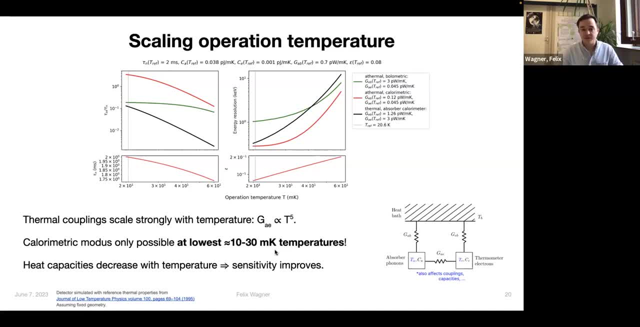 at these very, very low temperatures. This is the one and major reason why these very low temperatures are really necessary, And the other reason is that all these heat capacities, so in the electronic system the heat capacity scales proportional to the temperature, while in this photonic system 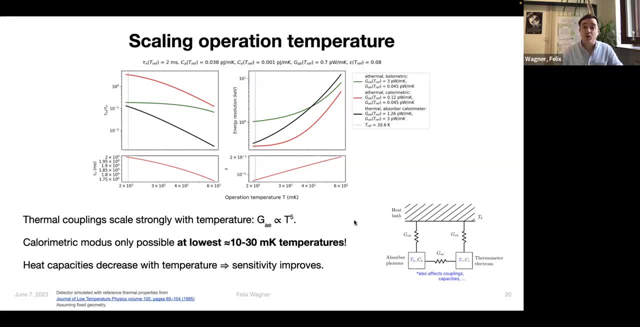 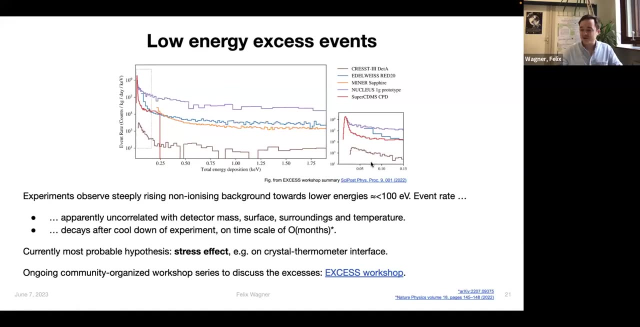 the heat capacity scales to the temperature, to the power of three. So in both cases we see that we we significantly lose sensitivity if we would operate these devices at a higher temperature. Okay, with that, already enough about the about the rigorous theory of these devices. 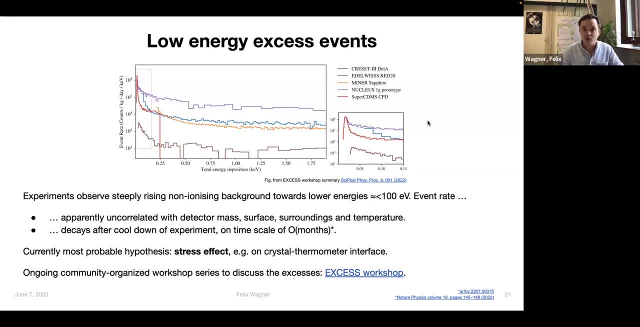 And I want to mention a couple of current research topics, namely: in the past couple of years, devices have reached energy thresholds of significantly below 100 electron volt And there appeared something that nobody expected And that is still a big, big question mark. 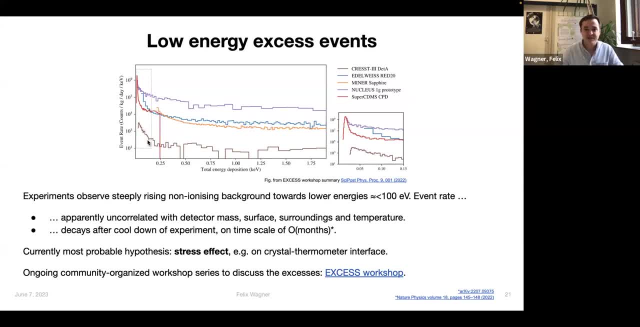 Namely a low, so-called low energy excess, And I put here a plot of measurements from several different experiments that all measure this phenomenon. Namely: this is an increase, a steep increase in the event rates towards lower energies, And currently the origin of this effect is not known. 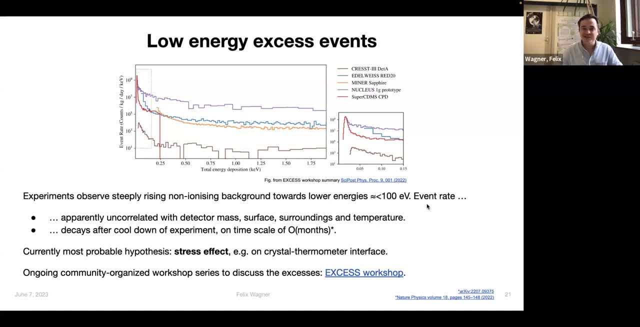 However, one could now kind of cheer and say maybe we found dark matter, but this is very, very well excluded the dark matter hypothesis to explain these excesses, Because this event rate appears at very different scales in different devices and has one characteristic that excludes 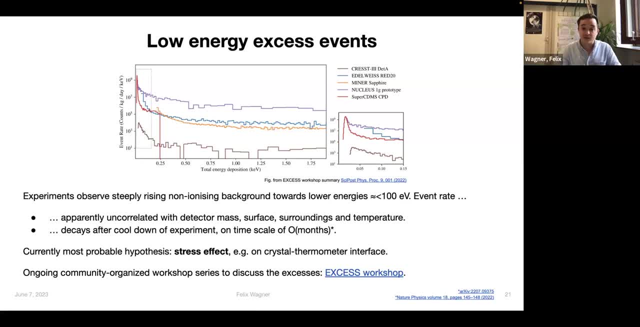 kind of excludes any external particle origin. Namely, it decays with the time of operation of the device on the timescale of months. So very likely this is a type of detector effect, But this is currently a limiting factor for the sensitivity of this. 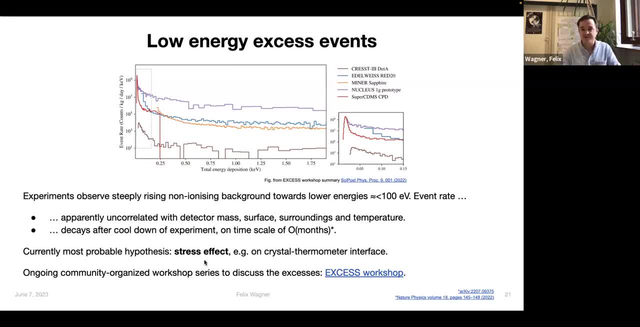 To explain these excesses is some stress effect, for instance on the crystal thermometer interface, And there is extensive research done to understand these excesses and manufacture devices that can, kind of you know, discriminate these excess events from actually expected. dark matter scattering. 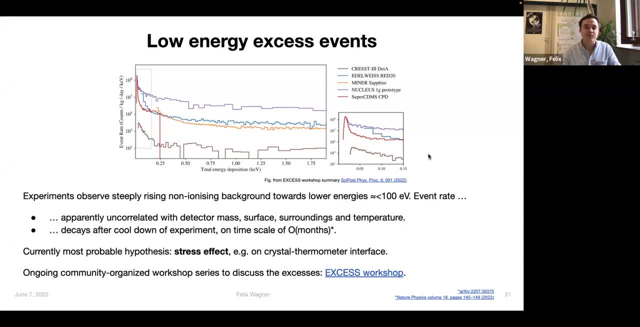 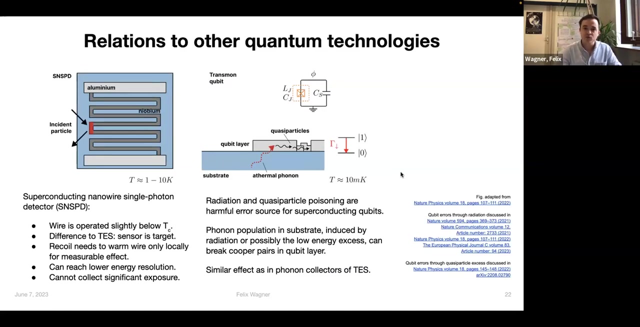 There is also a workshop that deals with these excesses, for a community organized workshop to discuss these observations. This is one of the very current research topics in this instrumentation And, before I conclude, I want to mention the relations to other superconducting and quantum technologies. 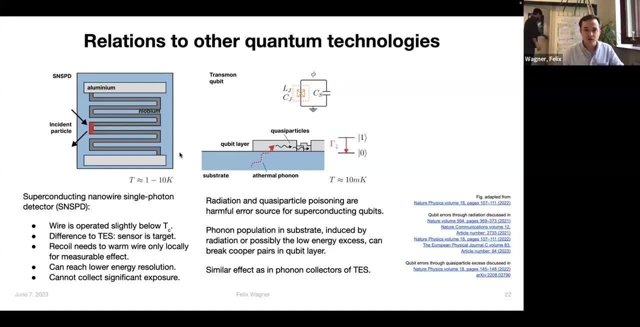 So if we compare now the superconducting thermometers to a different sensor type that is kind of prominent in this quantum technologies community, namely to superconducting nanowire CV-photon detectors, then we can find quite some similarities. So these SNSGBs- 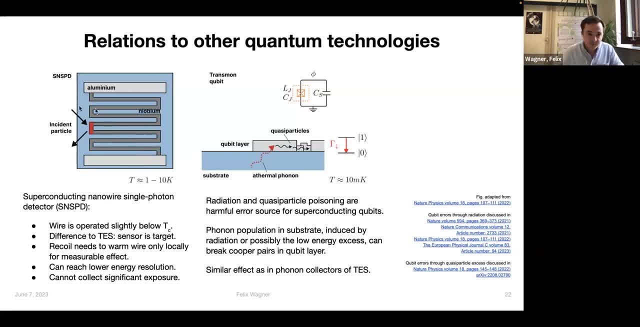 these are small wires that are that are deposited on some substrate And what they do is that if a particle recoils within this wire, then this locally heats up this wire, And the wire is operated similarly to the TS, very close to his superconducting transition. 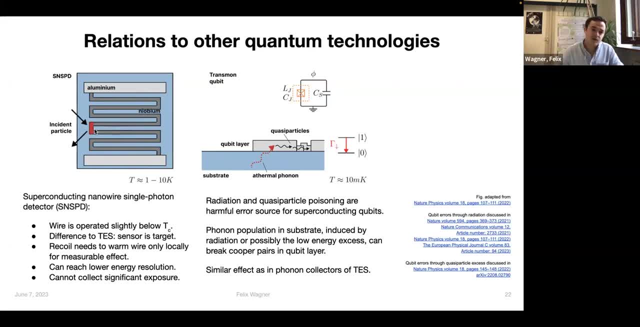 So locally, this wire increases, So the temperature of this wire is increased beyond the transition temperature, which again gives a, which is an effect that is again measurable, Therefore gives one a very sensitive device to measure particle scattering. The major difference compared to: 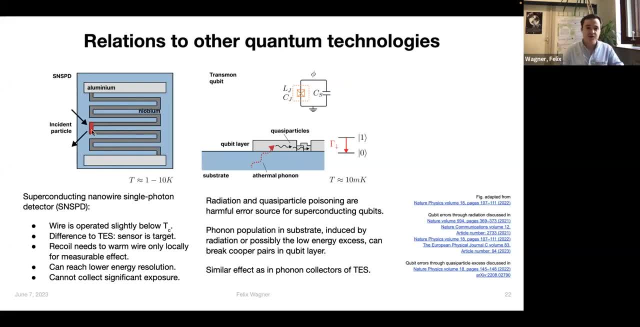 to the superconducting thermometers that are used for dark matter searches, is that here the sensor itself is the target. This can give a much stronger sensitivity, but also this limits the the exposure that can be collected, because this wire, of course. 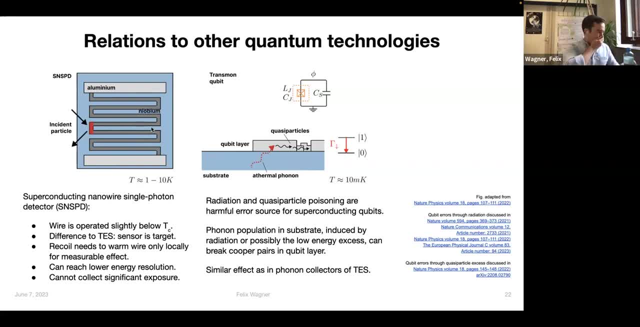 has a very low mass, I'm sorry. And the second connection to another type of superconducting technology that I want to mention is connection to superconducting qubits, also called transmon qubits, And an effect that is currently studied in these references that I put on the right here. 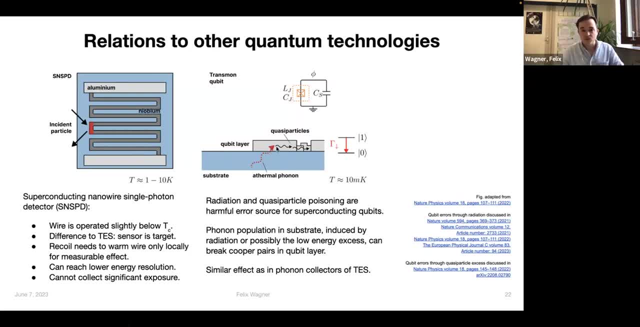 is, that is, to understand these error sources in superconducting qubits. And apparently one of these error sources can come from phonons that thermalize in the sensor and therefore break break quasi particles in the sensor And by that cause the decoherence and the error in the 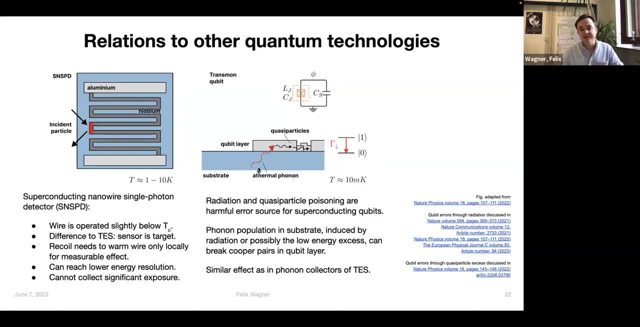 in the calculation of this qubit And this is kind of the same physics that happens for the phonon collectors in TES. This was studied in these papers here that phonons can can be produced, for instance from particle recalls or possibly also from this stress effects. 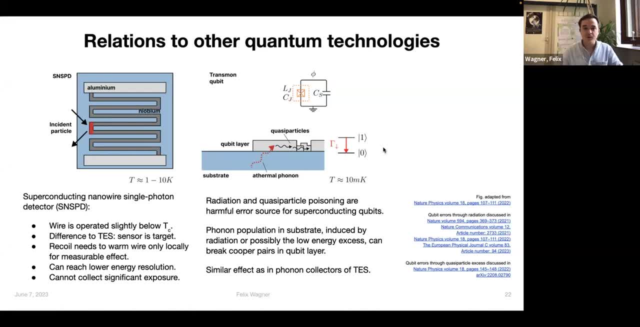 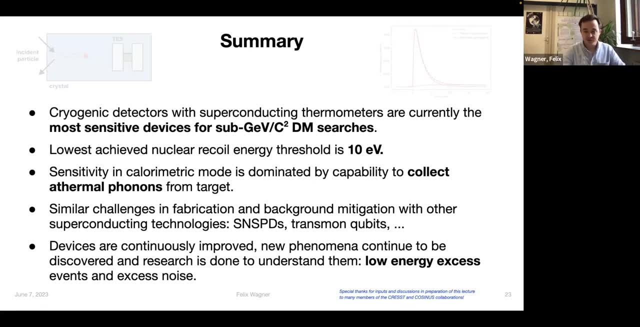 that we call the low energy excess. Okay, With that, I already want to conclude and reach my summary. Cryogenic detectors with superconducting thermometers are currently the most sensitive devices to measure sub-GUE dark matter particle scattering. The lowest achieved energy thresholds are only 10 electron volts. recall energy. 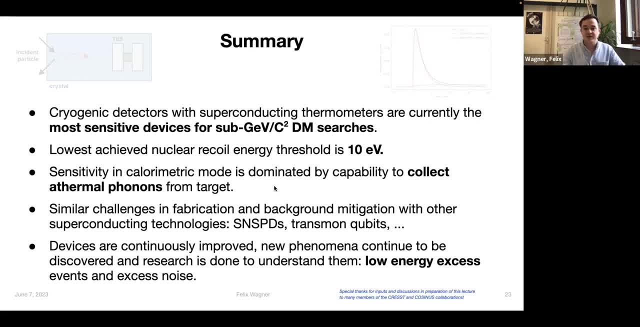 And the sensitivity of most modern devices is dominated by the capability to collect athermal phonons from a target twister. There are similar challenges in fabrication and background mitigations with other superconducting technologies, And these devices are continuously improved And new. 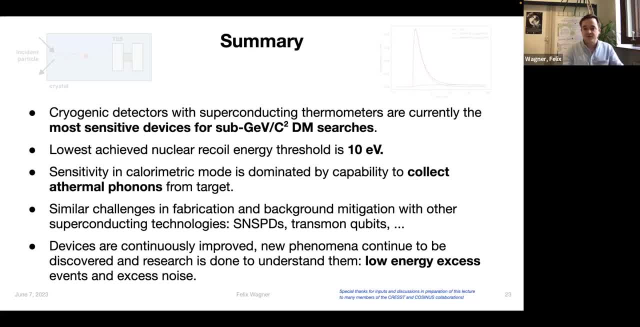 these new phenomena continue to be discovered and the research is done to understand them, For instance this low energy excess events. Okay, With that I'm done and I'm happy to take any questions now. Thank you very much. Sorry, I couldn't activate the volume. 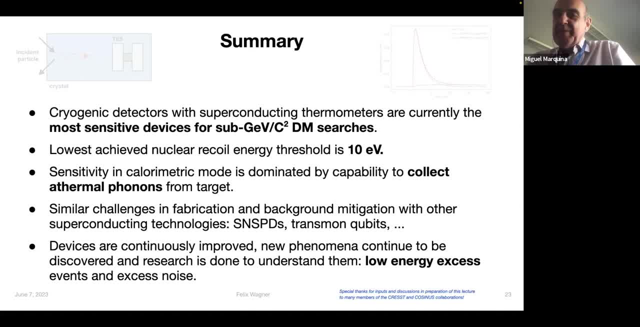 So thanks a lot. It has been very interesting really, for me personally, because I am a physicist as well, although I have taken some distance from this. So questions and comments from the people. You don't need to raise the hand anymore because you are already there. 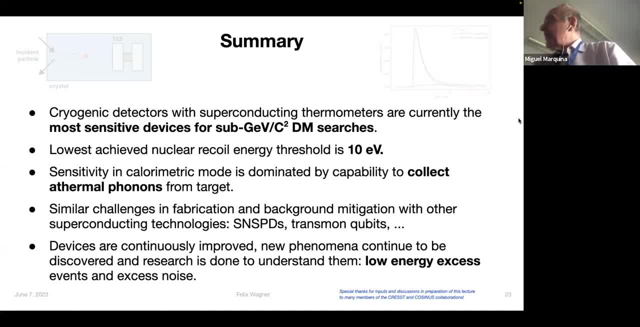 We are at the end of the actual presentation. Anybody who wants to start? Yes, Can you hear me? Please do Yes, Okay, Thank you. Thank you very much for this very nice and pedagogical talk. Okay, Very. 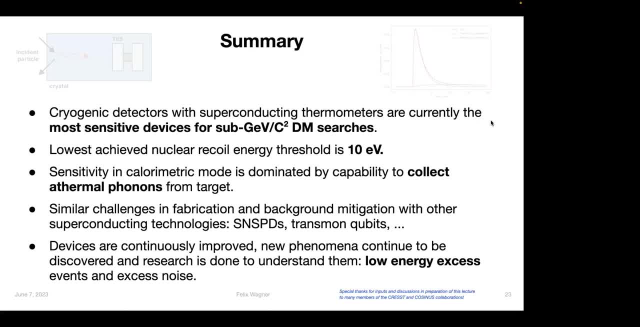 very clear, I think very clear and interesting. So I have actually a couple of questions. Felix, If I understand, one of the things that you have been showing here is the optimization of the different thermal conductivities between the bath and the and the. 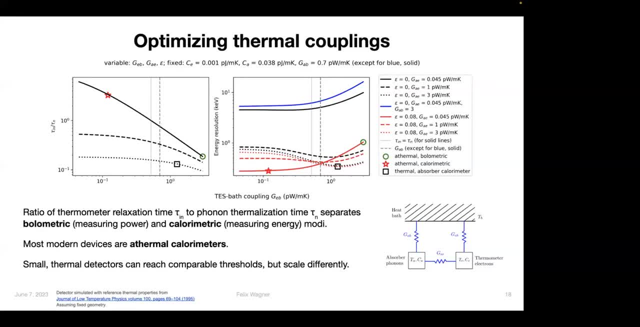 well, and the film that you put into the electronic system and the absorber right, The funnel system And, and actually you have, you are seeing here or you are showing here actually how, depending on these parameters okay, you may have different energy resolutions. 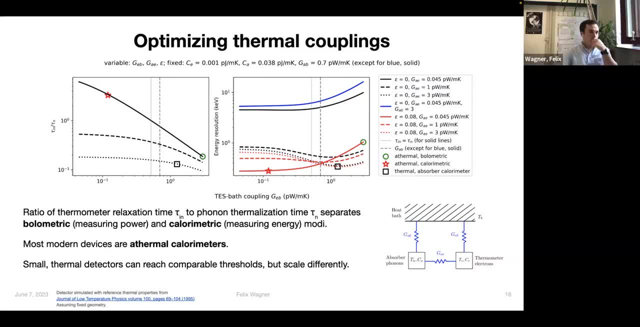 quite different, actually really different, Yeah, Okay, So the question is: how can you change or manufacture devices with different values of this for these activities? Because I mean, I'm I think this is kind of tricky. 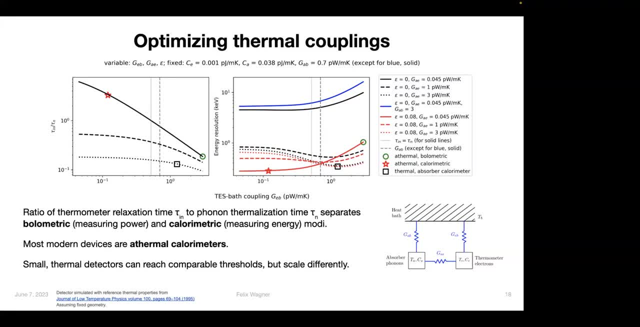 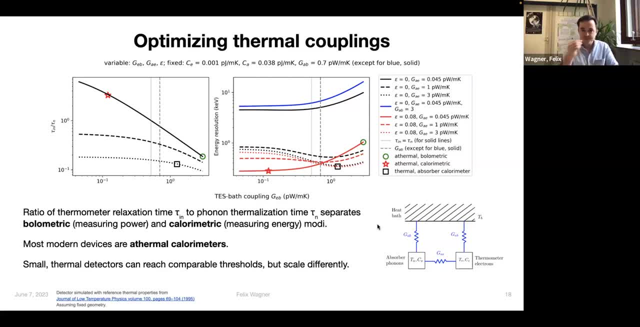 actually it is tricky, but there are ways to to do this. So the most crucial quantity here is actually this coupling between the sensor and the bath, And for that maybe, if I go back to one of the pictures of these devices. 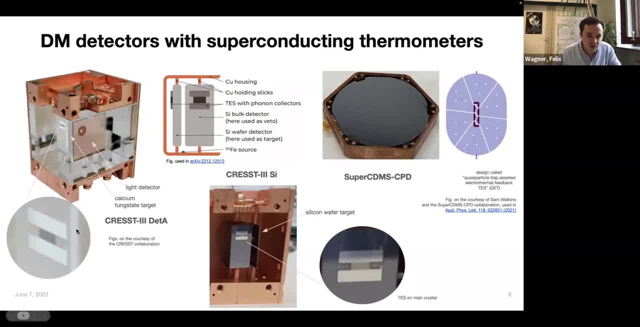 So usually this coupling has two major components, namely one is the, the gold bond, So the wire that leads from the, from the sensor, to to the, to the heat bath, And this you could. so the strength of this thermal coupling. 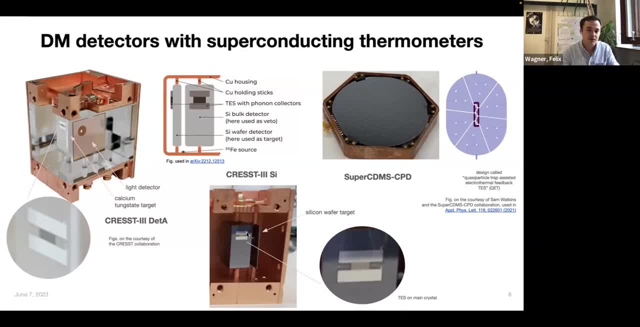 you could, for instance, so you you could put a ticker a thinner wire, or you could make the wire longer or shorter. But in fact, to reach this very, very low values of thermal coupling, you need to additionally have a technology to make the 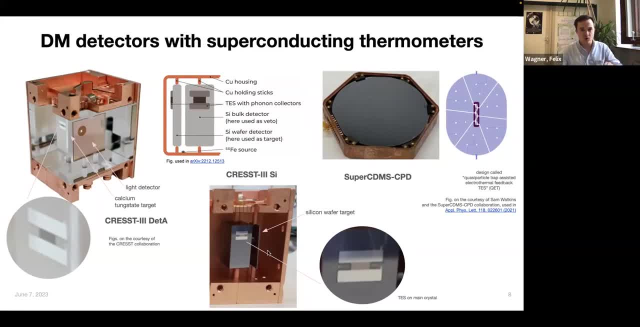 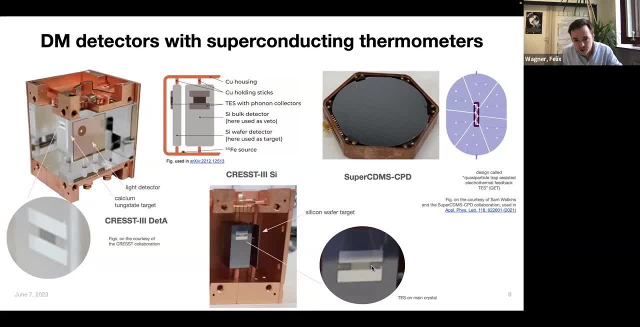 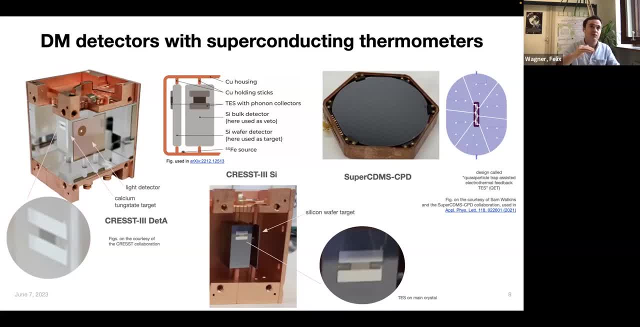 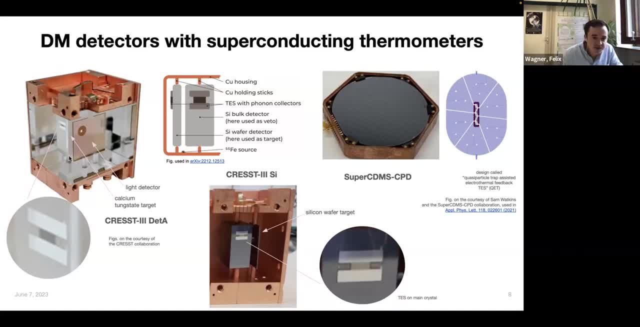 are um this: in this case it's- i think it's- a copper stick, uh, that holds the crystal in place, and so this, um connection between the crystal and the interface of the crystal and this copper stick that holds it in place, would be the point that dominates the thermal coupling from the crystal. 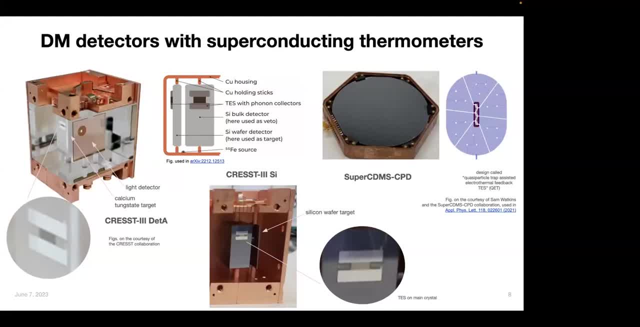 directly to the bath, and this you could change by, for instance, applying something, some different material for the holding or some different mounting, um, structure, um, and finally, the coupling between the film and the crystal is, at low temperatures, dominated by the interaction strength of um of the electronic and the photonic system, and this is something that scales with the 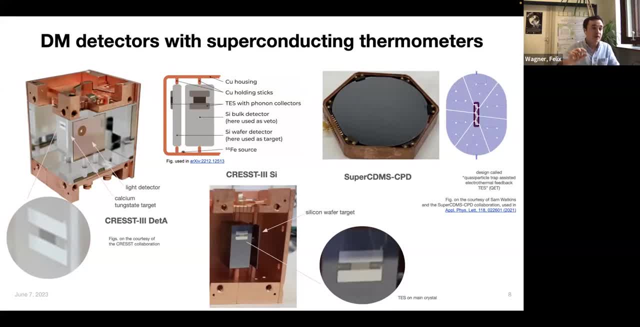 volume of the superconducting film and very strongly with the temperature. so mostly you control this by just trying to reach very low transition temperatures, which then um, which then makes this electron phonon interaction only very weakly and effectively reduces the strength of your thermal coupling. 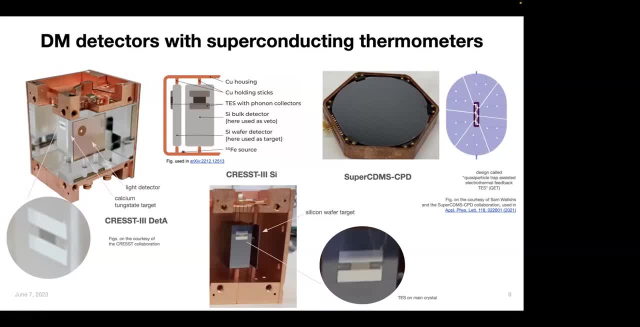 okay, okay, okay, thank you very much. this is, it was already. yeah, it's just going to. yeah, it's tricky, sounds tricky. right, it is tricky. yeah, that's what it looks like. okay, i only have time for another question which is related to that. or, yeah, go ahead, go ahead, okay. no, just to clarify one. 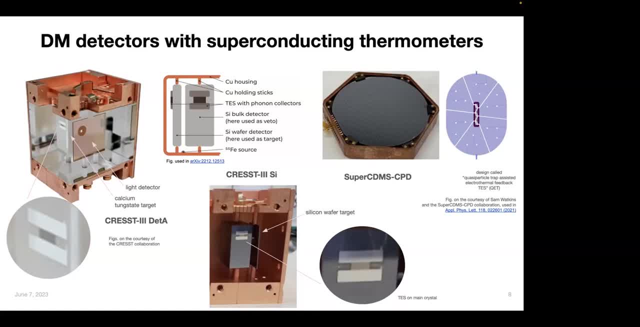 point, i think, because, um, you were mentioning uh a thermal, uh, let's say, but in, i think, if i understanding you, in two in two, in two exceptions, let's say in two concepts, because you were mentioning the, the, the direct detection of a thermal phonons, okay, those phonons, yeah, but also you mentioned uh a thermal. 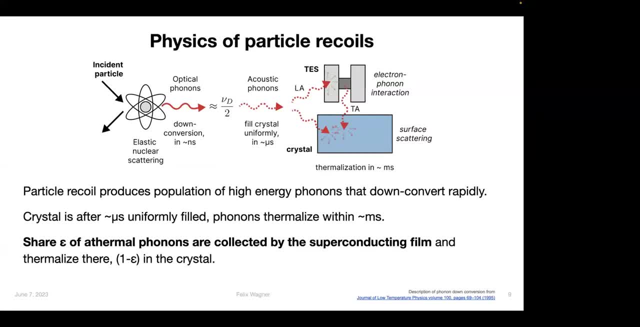 in the sense of um, just please correct me- in the sense that the actual, uh sensing element is: is the thin film right, the the capacity of the electrons and not the capacity on the phonons. okay, yeah, and then it wasn't clear to me, when you were saying a thermal calorimeter, to which one you were referring. 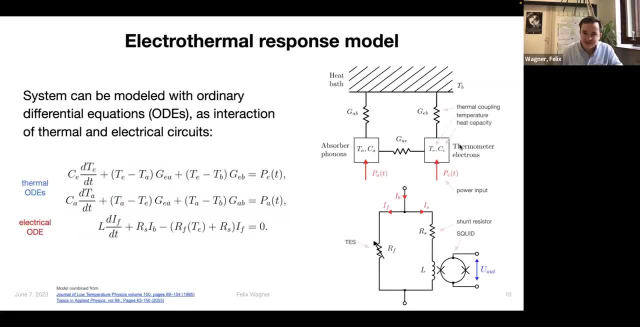 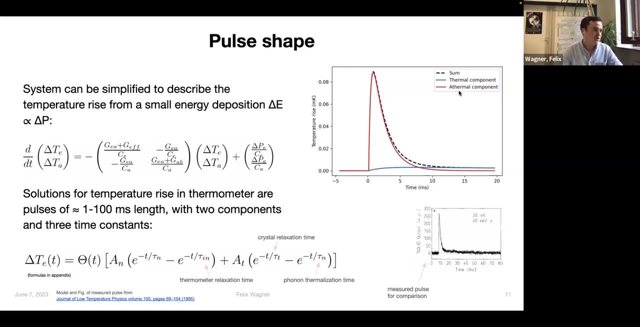 to. i mean it was unclear. yeah, um, okay, this is also a great question, so, um, actually it's okay. of course, everything that we measure in the end is temperature, so in the end, everything is kind of thermal, um, and what i mean by by this is a thermal calorimeter, and i mean it's a thermal calorimeter. 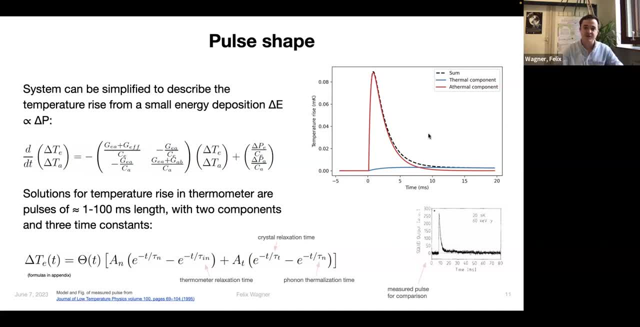 and the thermal component is that, um this compute, this component, the art thermal component is, but you is uh induced by our thermal phonons, so phonons that are much hotter than the, the typical phonon, um than the typical phonon. energy in the temperature, in the, in the thermal phonon. 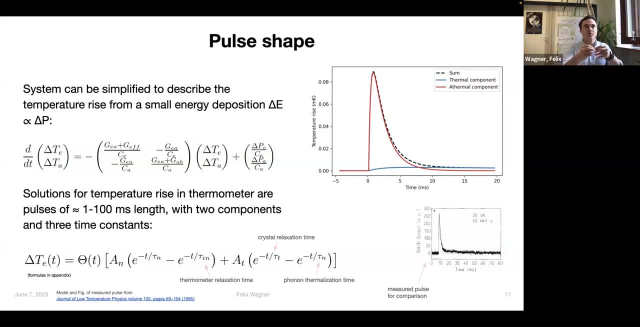 distribution um. so it's induced by this non-thermal phonons that scatter directly in the sensor and um induce a, so deposit the energy there and induce the temperature increase there. but of course it's in the end also a thermal in the sense that it is a temperature increase. 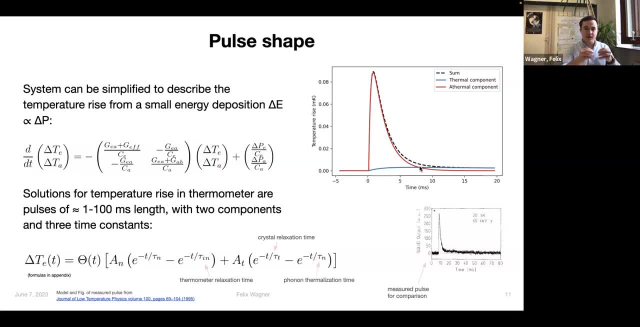 and and the other component is the one that really, uh, where the thermometer warms up because the the temperature, the actual temperature of the crystal increases, and this is why this is also called the kind of thermal component, because it's a really a temperature transfer one that you could. 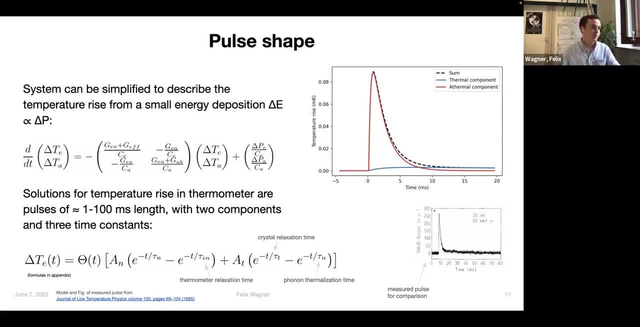 calculate, for instance, if the heat equation is the temperature of the crystal and the temperature has an observation as well. okay, okay, thank you very much. great talk, i, i love it, thank you, thank you, and uh, so somebody else? more curiosities, questions, comments, feedback? ah, it looks like not. 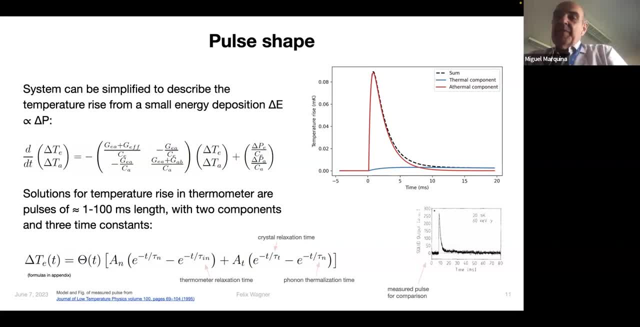 okay, so in that case, uh, before before closing, a well phil. thanks, felix. we cannot clap in a room, but feel like we are doing the equivalent. oh yeah, i see that in the icon. thank you, anastasia. so, um, before wrapping up, just remind you that, for those who just came,